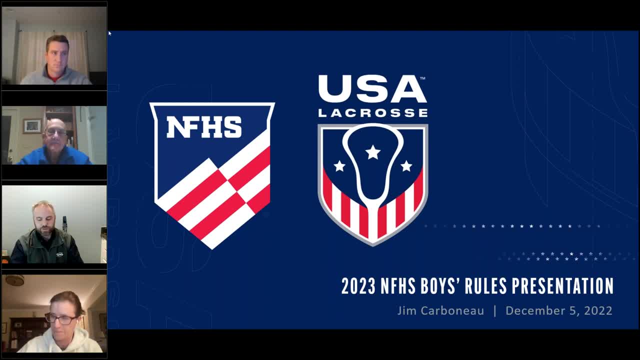 I'm the Director of Performing Arts and Sports for the NFHS and I oversee the rule writing process for boys lacrosse at the high school level. Mr Carboneau, Hi, Jim Carboneau, Mass, all up from near and around Boston. National Rules. 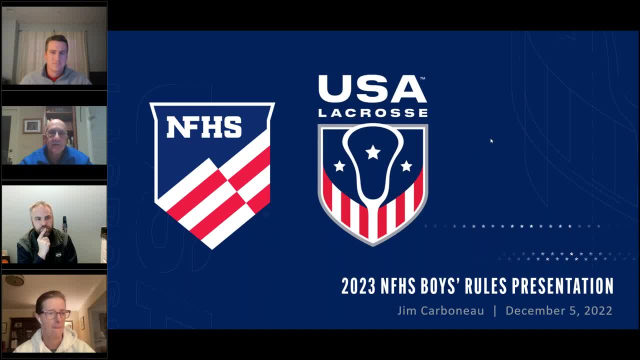 Rules Committee. I'm the Director of Performing Arts and Sports for the NFHS. I'm the Interpreter for USA Lacrosse for the 2023 season. So tonight's presentation it's going to go through a preview of the rules Jim and I have 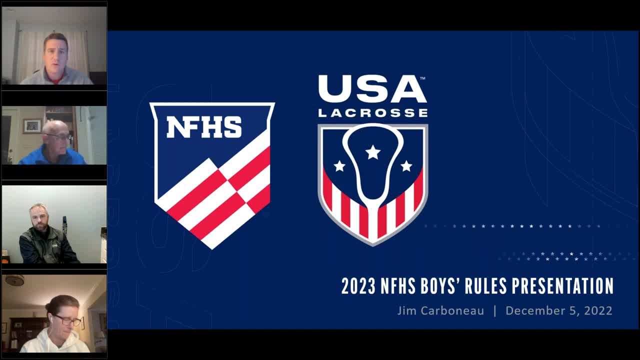 reviewed the press releases that have gone out in the rules books as well. If you have any questions, please put them in the chat box. Kaitlyn will be reading them and then trying to filter them in as they come along If we don't get to them. hang on to the end of the 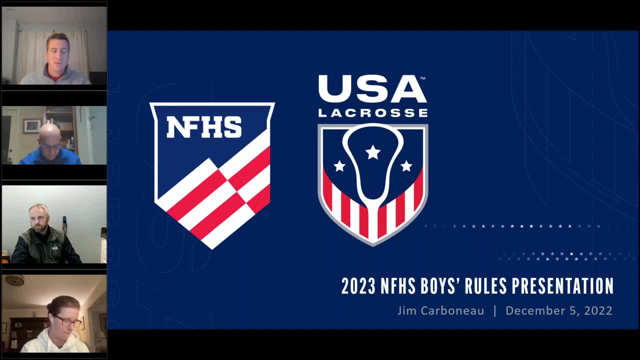 presentation and we will try to get them the best we can. What we typically do is try to take all the questions from here and then include them in a future presentation in January, which we'll then try to distribute online. So if there's any corrections or 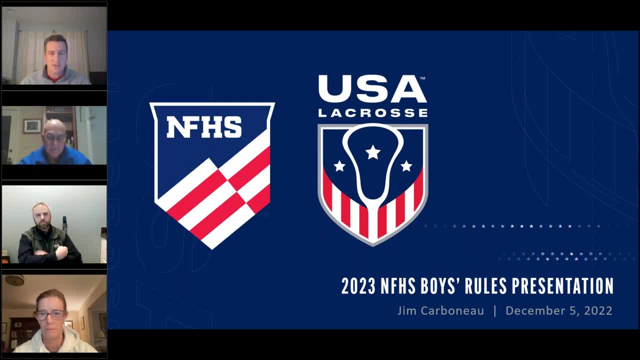 if there's any new information that comes out from this, it'll probably be part of this presentation. Kaitlyn and James will release that information to everyone, so they have that for the start of the season And, yes, I hope that we're able to get this out for. 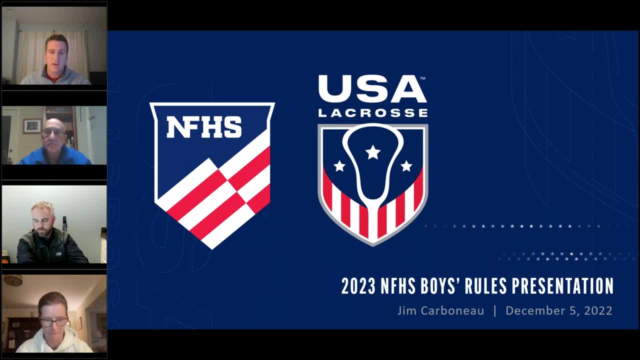 our warmer weather clients or, excuse me, our warmer weather folks in Florida and Texas, who start the season right away. So, without further ado, we're going to go ahead and jump into things. James, anything you want to say on behalf of the NFHS before we get started. 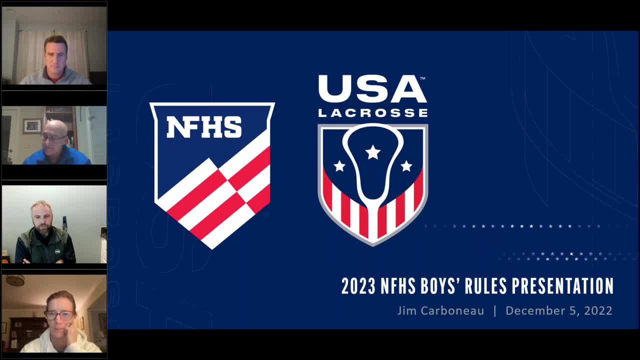 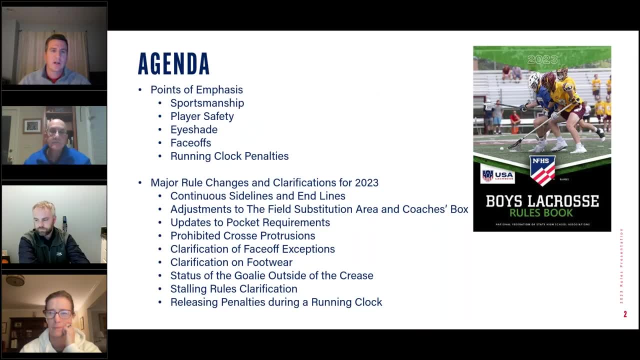 No, just. we appreciate the good working relationship we have with USA Lacrosse and we're looking forward to a great upcoming season, Thank you. So today's agenda: we're going to cover the points of emphasis, along with the major rule changes and clarifications. 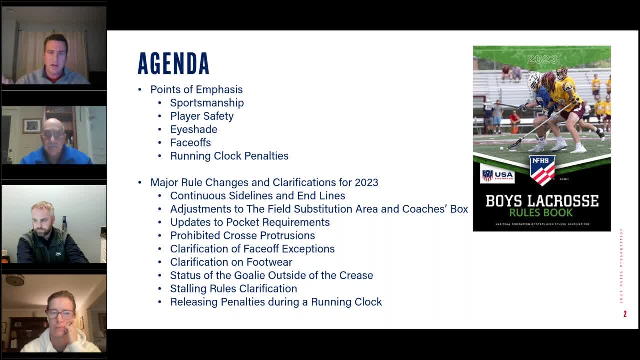 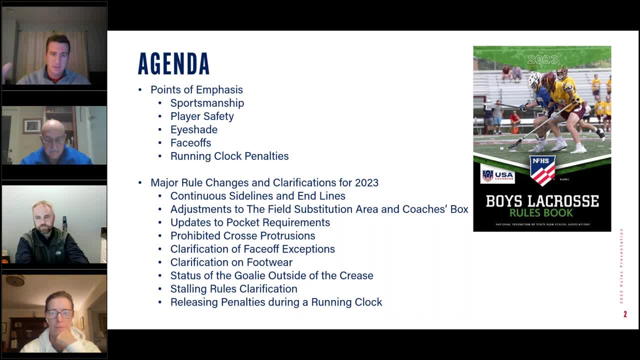 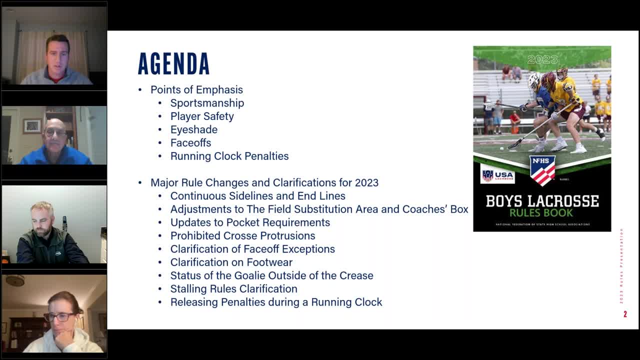 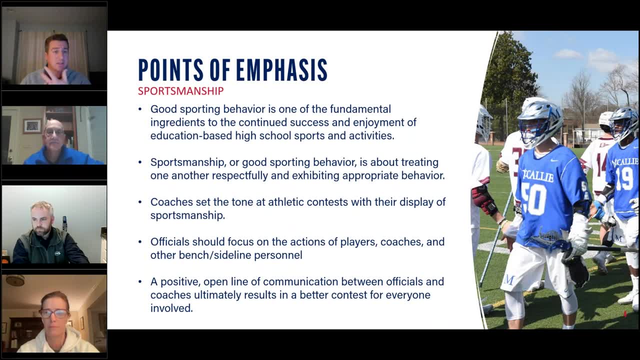 as you take this to your coaches and officials across the country. So again, any questions, please put them in the chat box. So points of emphasis. Jim, do you just want to cover briefly sportsmanship? It seems like it's something that we have each year, but it's. 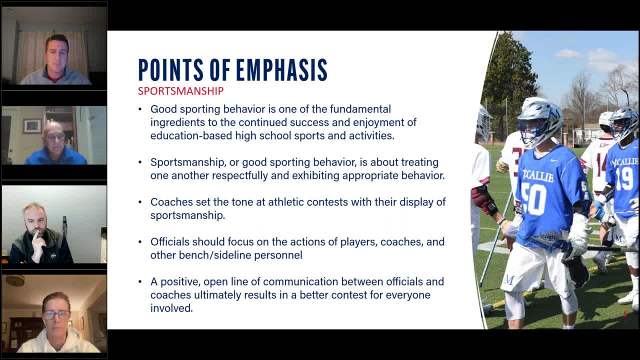 always an important thing that we want to make sure that we convey the relationships that we have for you on the field, know the relationship between coaches and officials. yeah, i mean, it's obvious, um, we see it every day, in every venue, in every sport: that sportsmanship is being uh driven by the wayside. 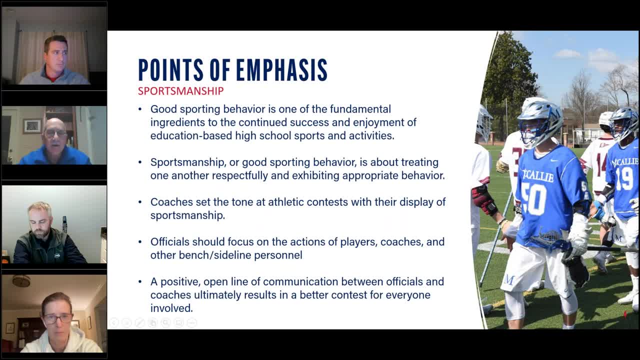 and we feel at usa, lacrosse and the federation, and we have to make an emphasis on it and um and, and we're going to make the emphasis on it with ourselves by making sure that we do everything, we do right, we do it professionally, we come in with the right attitude. 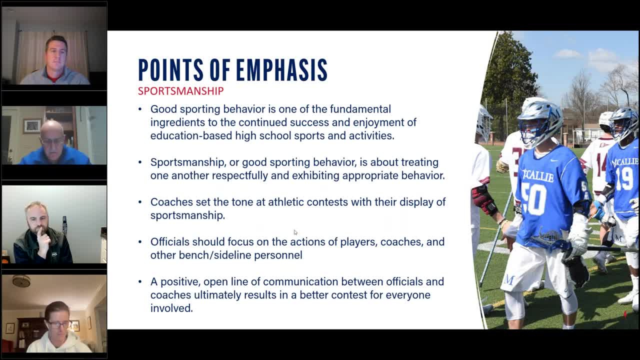 we've all been yelled at by by coaches, we've all been harangued by fans, so on and so forth. we've got to keep the the stiff up the lip, be classy, be positive, make sure that our communications with the coaches and the um the staff. 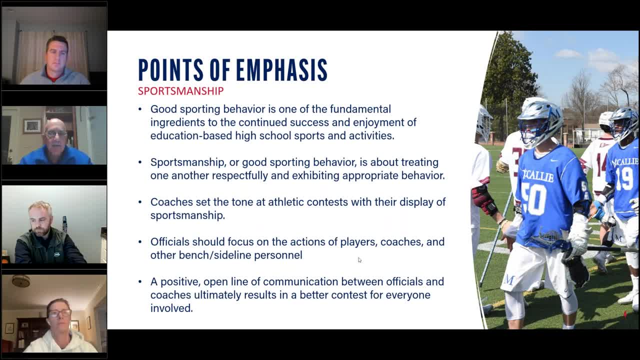 uh, uh are fair, firm and in the best interest of uh of the games, and it's just an emphasis for everybody. uh, we're going to try to get working with the coaches and and the adults, as, as the adults are the third team on the field in working for the, for the good of the kids, especially at the. 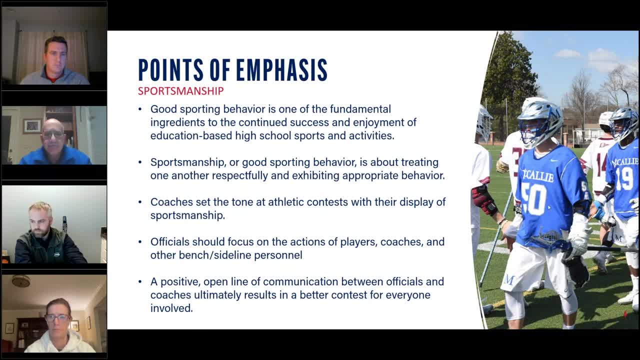 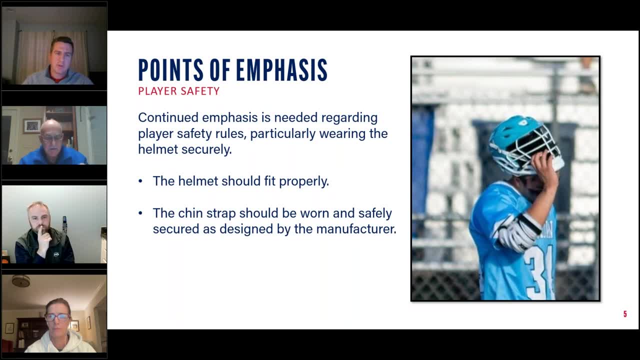 youth level, but also at the high school level too. thanks, jim. okay, points of emphasis: player safety- um, i'll go ahead and jump in on this one. uh, players equipment and how it's worn properly is, uh, something that we all need to be cognizant of. so i think, um, this is sort of self-explanatory, and 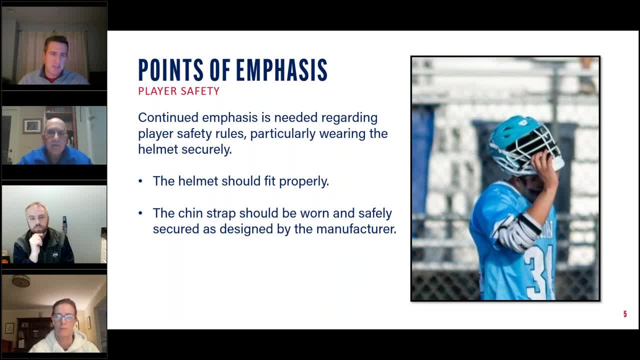 something that's sort of brought up. all the time the helmet needs to be worn as it was intended by the manufacturer, and all four points of the chin strap need to be worn at all times, as you can see here. uh, sometimes a fully strapped um helmet is pulled off by a flavor that means it's not being 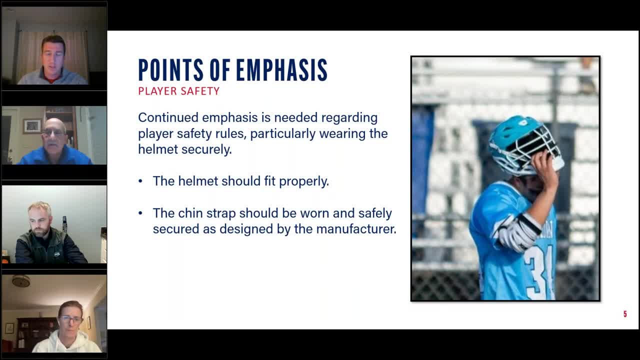 worn properly, because if it is worn on properly, it can't be removed. so, uh, make sure the players are wearing their helmets safely. uh, that goes for coaches to talk to their players about it and officials, uh, to talk about that um, in their pre-game meeting with coaches. um, eye shades, um. 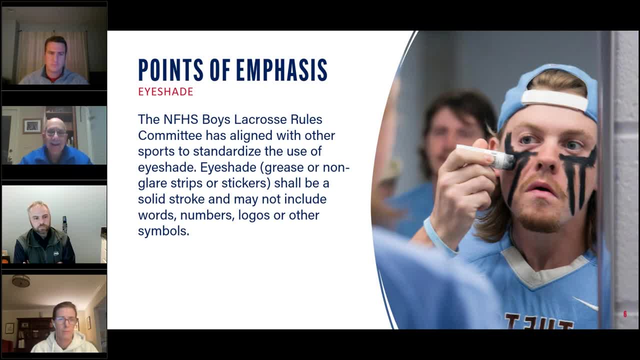 jimmy, do you want to go ahead and take this one? uh, it is what it is. um, you know the high schools and the federation. uh, and every sport has said that eye shade should just be the single line. uh, one of the issues we've had in the past. 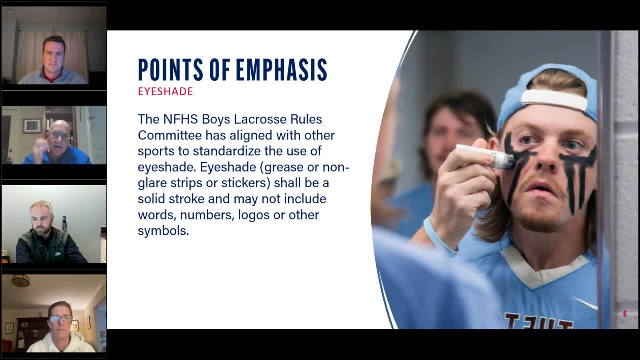 is, um, people writing offensive or negative things on the, the eye, the eye shape and so on, and we just want to curb that. um, it is what it is. if we started early and make sure the coaches and players know in preseason and reg at the beginning of the games, uh, it'll be something, it'll be taken. 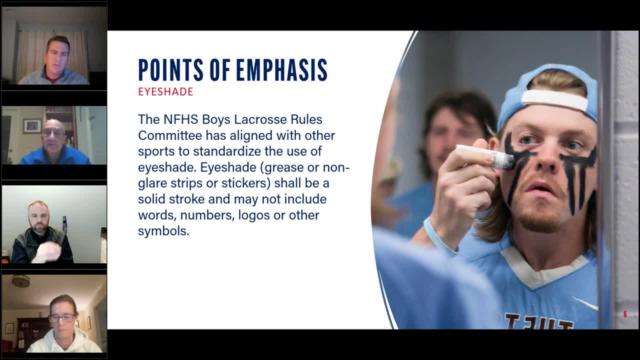 care of- and- uh, james, correct me if i'm wrong- this is a uniform uh rule for all high school sports, so it's not like lacrosse is being picked on in particular, correct, correct, yeah, and this is something that's being used in football, baseball, um points of emphasis, i believe, is in all of those. 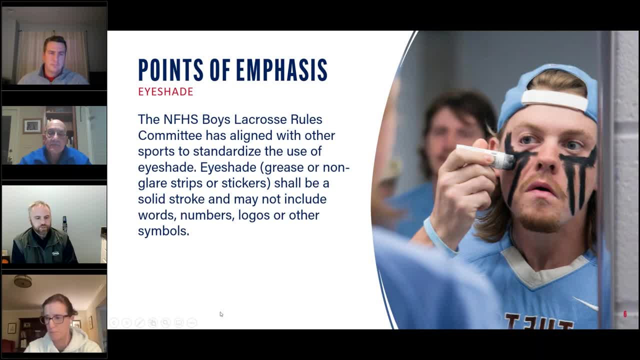 um, and the whole idea of it, like jim was saying, is just to make sure that we're using eye shade for the reason it's supposed to be used and not using it for any intimidation factors or anything else. one thing that the rural committee wants to ensure is that we can't tell the people what 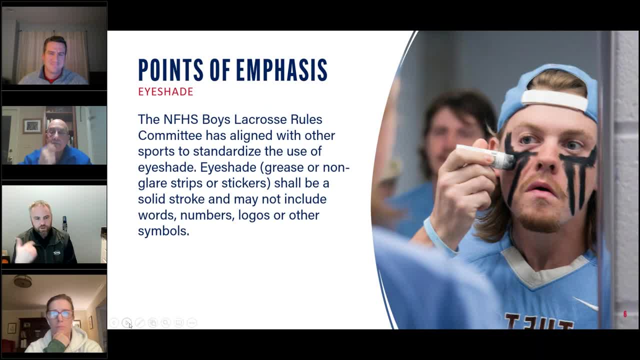 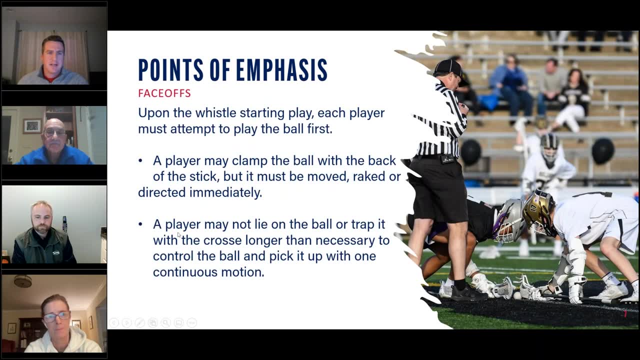 may or may not be offensive, so just know that one solid stroke is what it's supposed to be. great, uh, face offs. do you want to go ahead and talk, um jim, about the face off? there's a lot of evolution of the face off and a lot of things happened in the past few years, from the 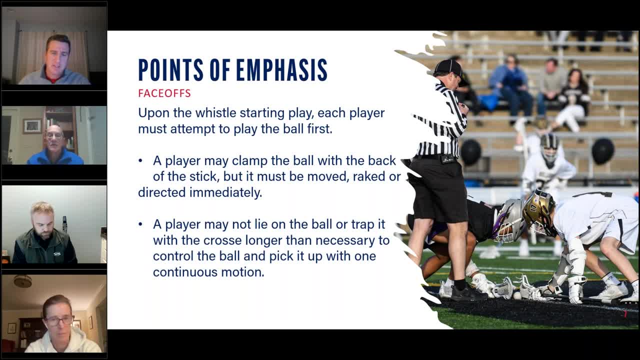 college level all the way down to youth. but do you sort of want to, you know, summarize, um, you know what the, the general pulse of the lacrosse community is on the face offs and, you know, touch on some of the things that we'll be doing a little bit of a deeper dive into in this. 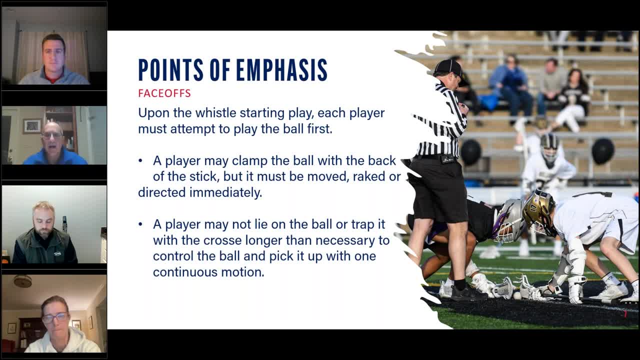 presentation. yeah, the most important is get the ball out of the area quickly, either in a stick or out of the scrum area. um, the point of emphasis: uh, you have to play the ball first. you cannot dive into and hit the player with, uh, with the right hand or with the left hand, or with the left hand, or with the right hand or with the left hand. 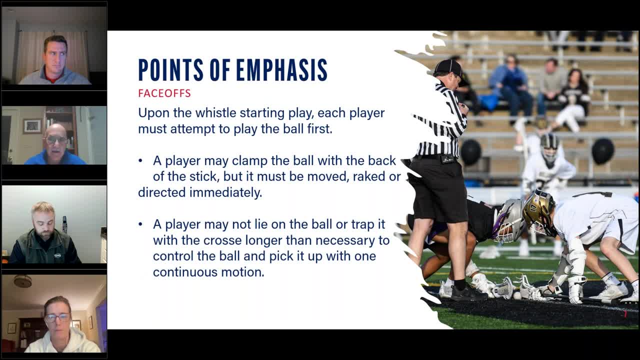 you may clamp the ball, move, rake the directed immediately. now we've discussed what immediately means and it's within one step. it's what's been promoted at the college level, the pro level, and and forcing it and making sure it happens at the high school level. if it's clamped, if the kid looks up and looks around. 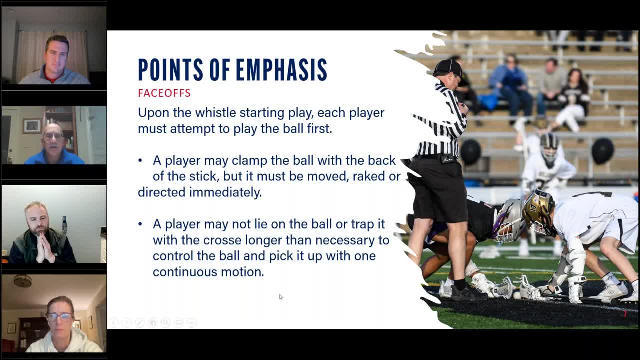 it's a take the ball away from him. it's not immediate. he's com, he's controlled it and he hasn't moved it. it's a clamp, step, drag, pop and same thing. we may not lie on the ball or trap it on the cloth. trapping in the cross is where i said he clamps. it looks up to see where his players are, so he. 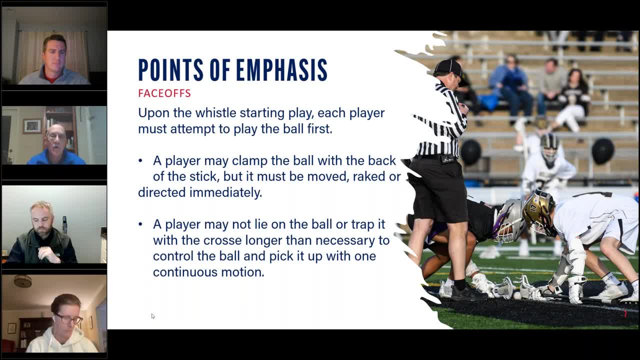 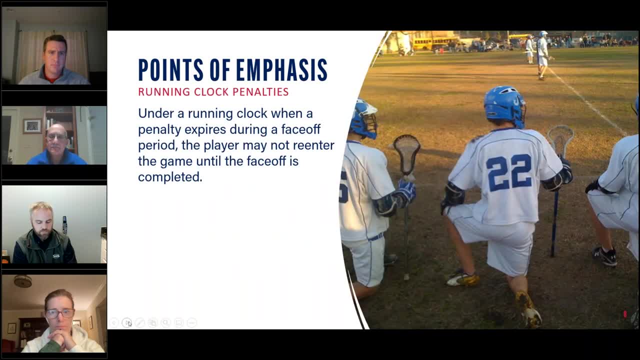 can direct it to them. if he does that, he's, he's withholding. it's clamp, drag, pop it out. right, um, i'll take this one running clock penalty. so, um, under a running clock, when a a penalty expires during a face-off, the player is not allowed to re-enter the game until the face-off is completed. 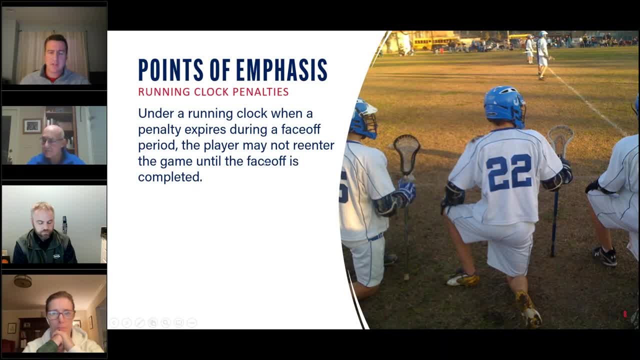 uh, it's a point of emphasis because it's a finer point of something that does happen in game, so we'll- we'll dive into this a little bit later, but that is one of the points of emphasis from the committee to make sure that this is discussed by officials and coaches so that it's well. 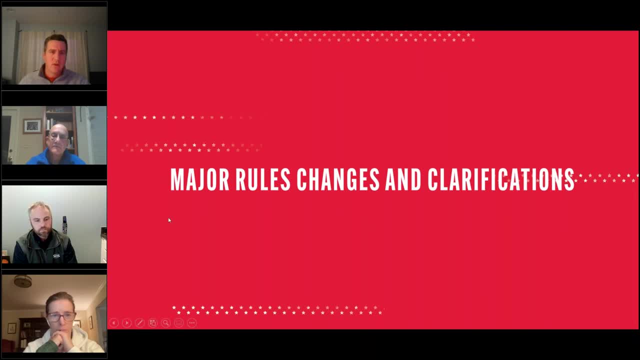 understood when it occurs in games. so with that, we're going to go ahead and jump into the major rule changes and clarification. we're going to go ahead and jump into the major rule changes and clarification. we're going to go ahead and jump into the major rule changes and clarification. 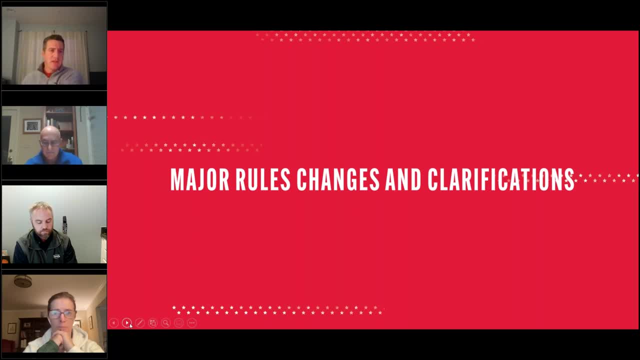 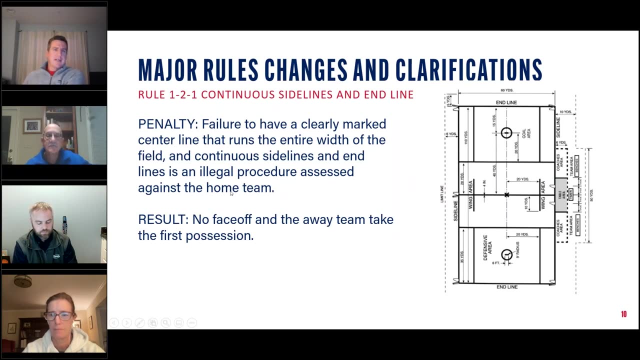 this year again. any questions, please put them in the chat box and caitlin will interject when she has a chance. um, rule number one, jim. uh, do you want to talk about? um, the? uh, i guess that sort of the, the clarification of continuous sidelines and end lines, maybe what? 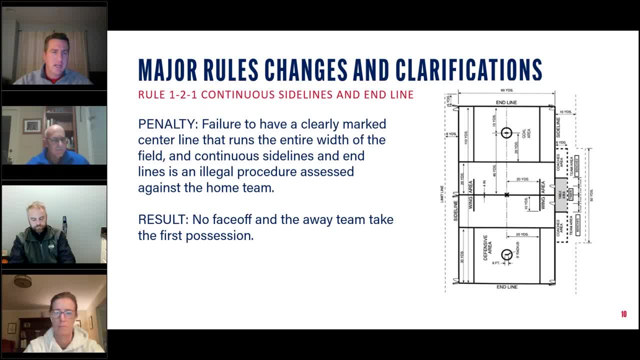 we were seeing out there on existing fields, and then how it's handled from a penalty perspective. i know this is one of the questions that was asked. how often can it happen? when is it addressed? and you know what are officials supposed to do? um, you know, when they walk up to a field that is uh. 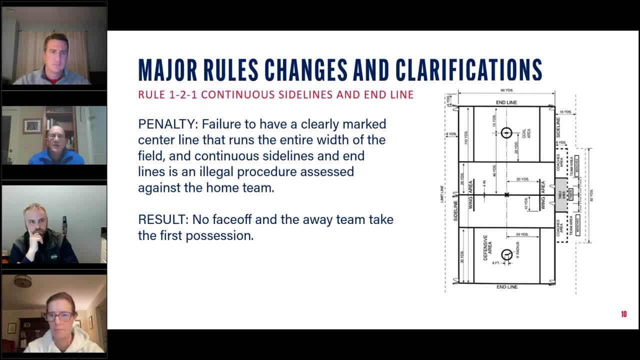 improperly marked. yeah, for years we have. we have not addressed the situation because with with the idea of growing the sport and getting more and more people going and um with the, the emergence of turf fields everywhere and there's only certain amount of lines on on turf fields, and especially if it's a football field. 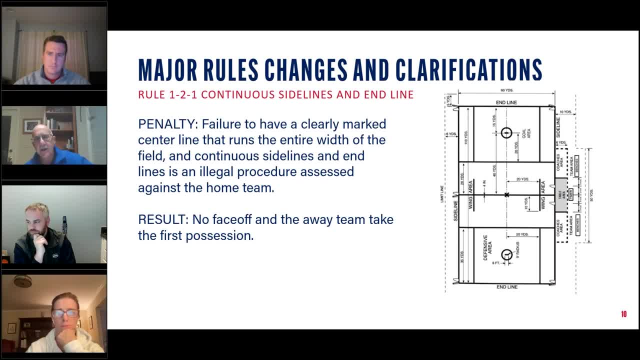 then it's just not a sport. that can be a conversation. uh, we have always kind of let it slide, but but uh, the field has always tended to be a very progressive field and we've always let it slide and we've always kind of extended lines, so on and so forth, and we've 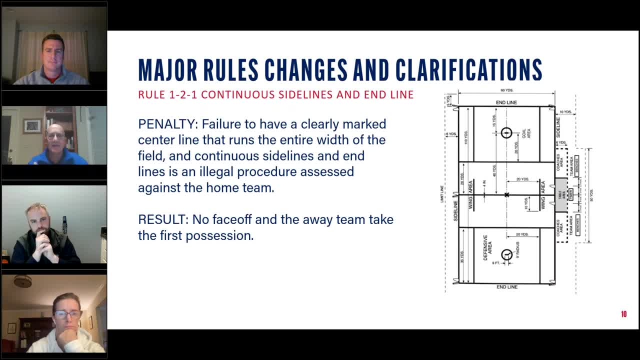 always kind of let it slide. now that lacrosse is becoming more and more mainstream, i think we we can ideas of doubt: was it over the line, wasn't on the line, where is the line? so on and so forth. so this is a nudge, a push to get the clearly marked fields: 100 sidelines, end lines and 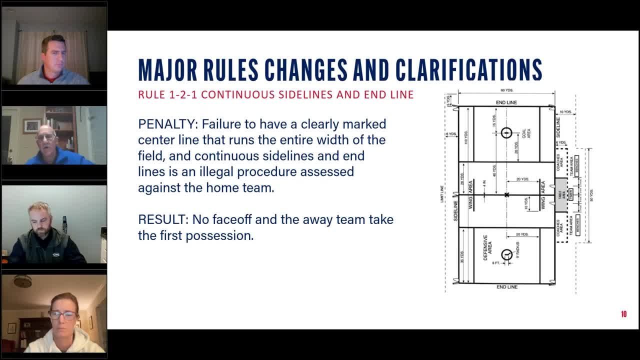 the penalty is much like it was with the midline. it's just simply loss of ball on the first possession. it's a push to get everybody to do the do the field lining correctly and now that we have the paint that you can put the temporary paint and it washes off in a in a week or two or 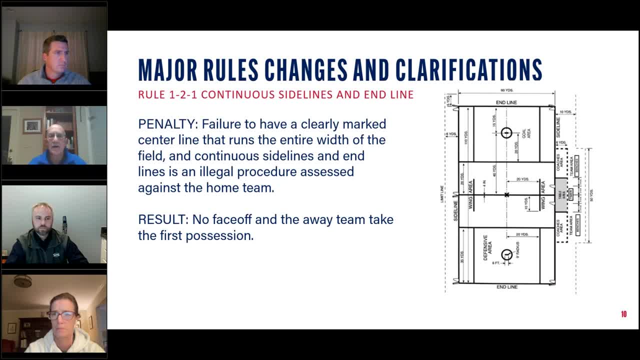 a rainstorm. I know football coach is going to lose his mind that we are tarnishing his field when his football team comes on it. so we're looking at making it a full field and complete this year with this. with this push great and one of the other questions. 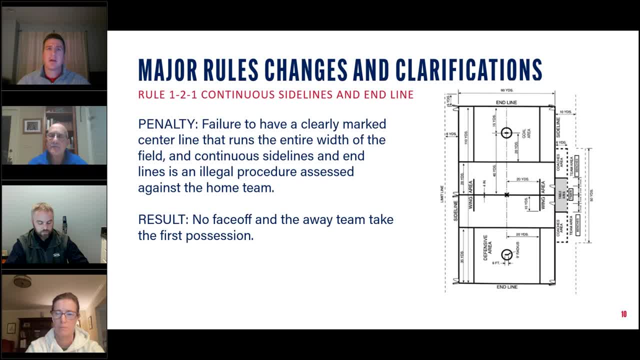 that came in about this too, is: how many times per game can this penalty be enforced? just the opening face-off, just the opening face-off. so only with the opening face-off, not in the second quarter, second half, overtime, none of that correct and correct. and, and in some areas, in some areas, local. 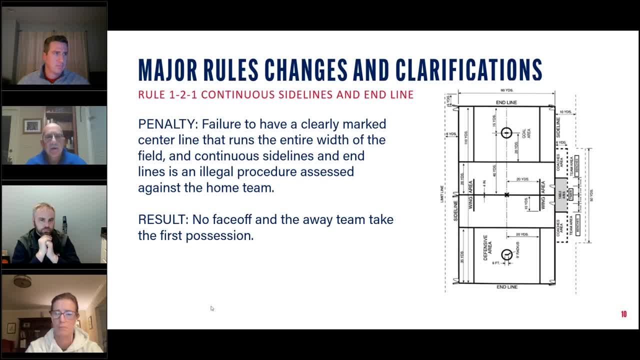 high school people in Massachusetts. they've waived certain rules and it's sometimes this rule might be waived by your local. so make sure that if your state organizing body is it is in agreement with this, you you make the call. if your organizing body has waived this, then it's not your call to make Caitlin, do you? 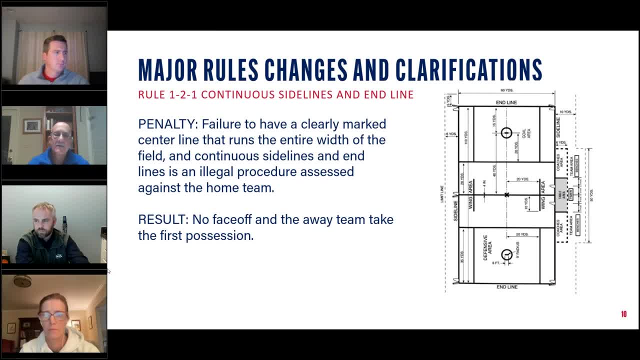 want to go ahead and interject with maybe, some questions that have come up. sure, I didn't know if you wanted to keep them for the end or go back, so, James, I'm gonna throw these questions, I think, to start to you. the first question is around the eye black and just asking: how are other sports handling eye black, since you? 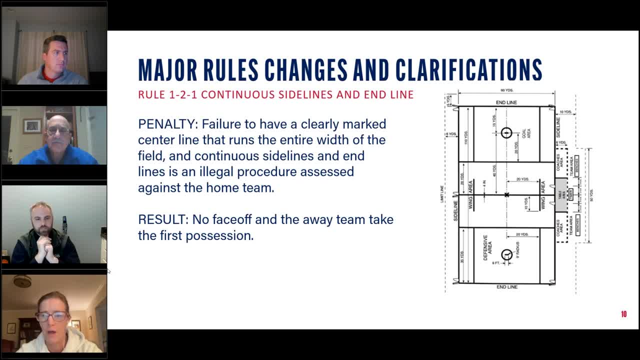 know teams do seem to violate this point of emphasis and the the person asking is saying is concerned that if they do it in pregame it will set a bad tone from the beginning. I just didn't know if you had any guidance from other sports. I will say in the women's game this has been a rule for. 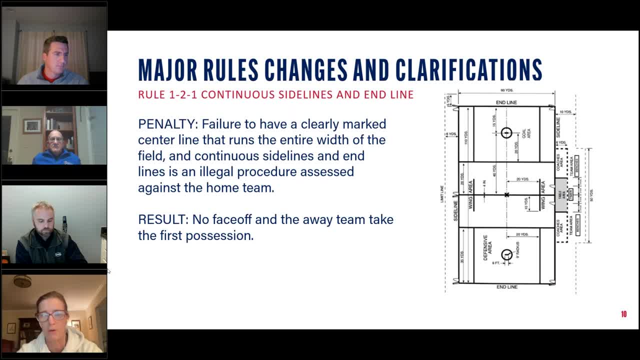 multiple years and we remind the coaches in our pre-game, when we ask them if their players are legally equipped and in uniform, that that is part of it and it's been a pretty established thing at this point on the women's game side. yeah, and the eye black rule has not changed in the boys. 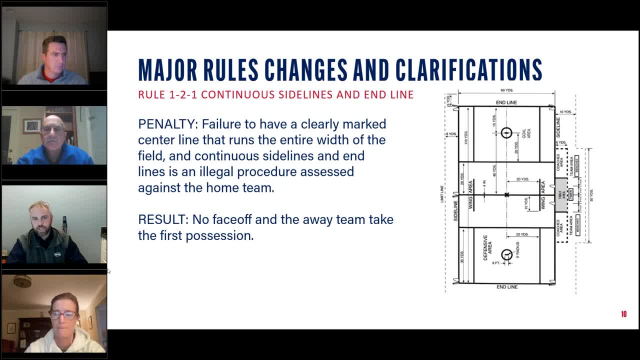 games. so the penalty, the expectation, is all the same. it's just a matter of making sure that's an emphasis, so we avoid kind of having that, um, you know, war paint style thing being put on your face, um and so. so nothing has actually changed for us and it should be addressed in the pre-game, because 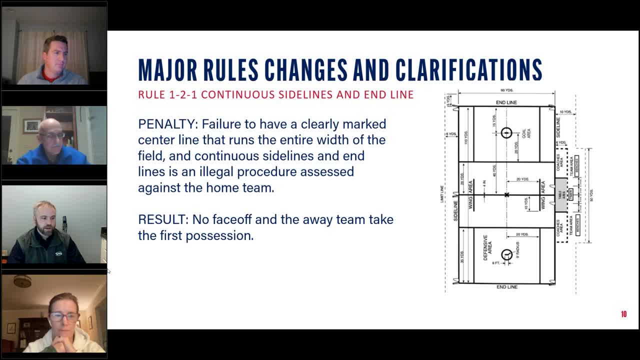 you don't want to have it on during the game. so during the pre-game, uh, all the pre-game mechanics. this is when that should be addressed. there's no bad tone. go, wash your face, put one swipe on, move along with the game. and the second question is also about a poe. um says you know sportsmanship. 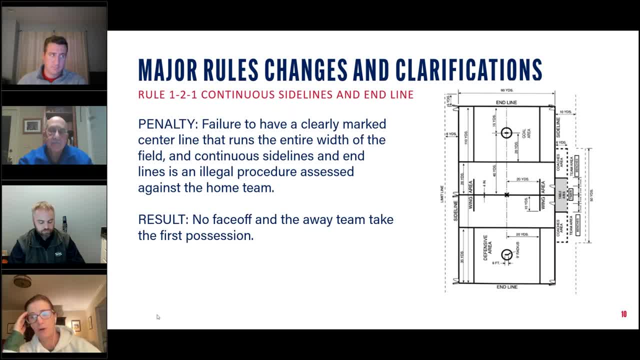 has been a poe for several years. what can be done or is being done at the state and local levels to communicate um to the coaches, etc. on that topic? so the uh, the nfhs and all sports has started this campaign called bench bag behavior. uh, it is. it's going to a lot of tools for the state associations. 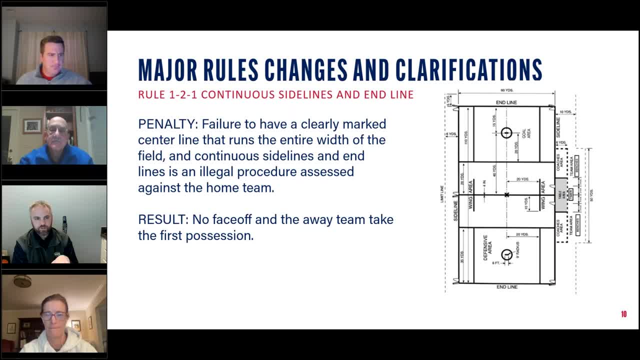 to use, make sure that our friends at us, the state associations, are using it to make sure that our friends at us, um, but this is something that is not just a lacrosse issue. this is a across the board in every sport issue. uh, sportsmanship's a thing. it's gotten worse. 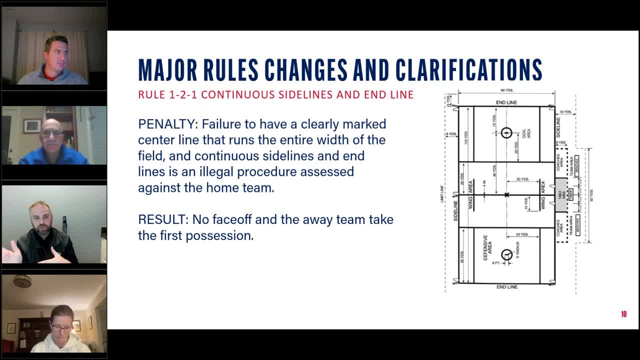 since the pandemic, um- and it's really become fan- behavior has gotten worse, which then causes different sportsmanship issues on the field, um, you know. so i just people just need to remember like we're all humans, let's be nice to each other and then just go play a good game. 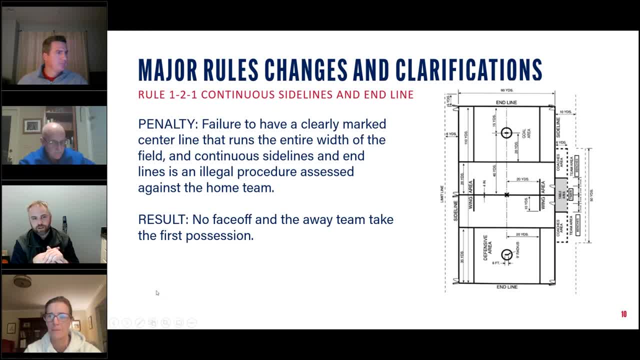 um, but i think there's a, there are some are some things that we need to be doing, that are some tools being created. i know us lacrosse has a lot of uh resources on um sportsmanship, as well as the nfhs and the ncaa. so i would say, use those resources to the best of our abilities and then 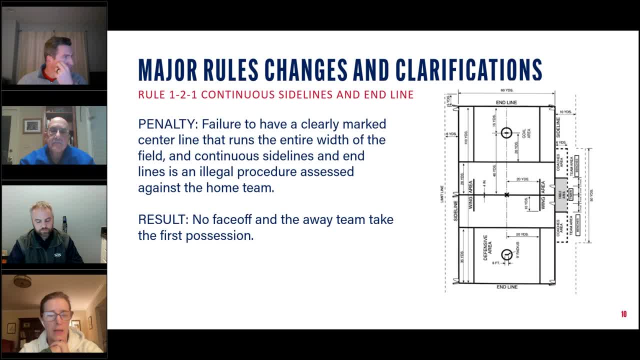 one quick follow-up question: what penalty should be used if the eye black is not addressed? oh shoot, let me grab my my rule book here. hold on, do you think i have that ready to go? but i don't. i will answer. i can answer it back in the chat box so everyone can see it. 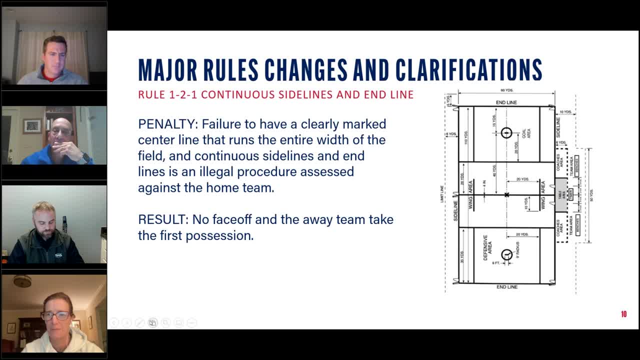 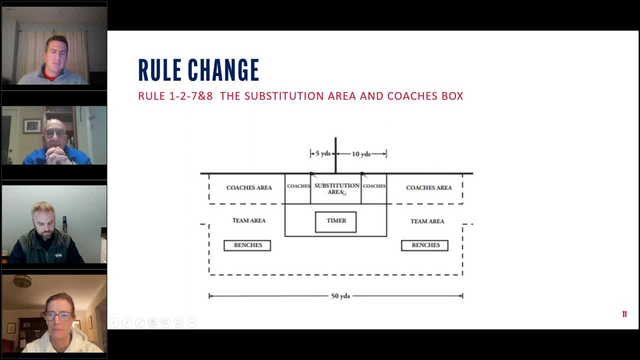 afterwards. if you guys want to move on, sure, all right. moving on, um, a little change, uh, the substitution area in the coaches box. um, jim, do you want to sort of talk about? uh, you know where the changes are and then, um, i guess maybe what they were changed from using the illustration we're 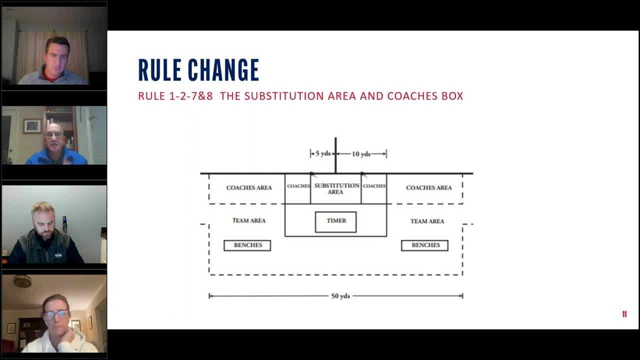 looking at here on the screen. yeah, uh, the last few years the substitution box has been 10 yards on each side of the the midline. so if it's a football field it's from the 40 to the 40.. um, now this year they're shrinking the box back to what it was, uh, from 1950 to whenever we changed it. 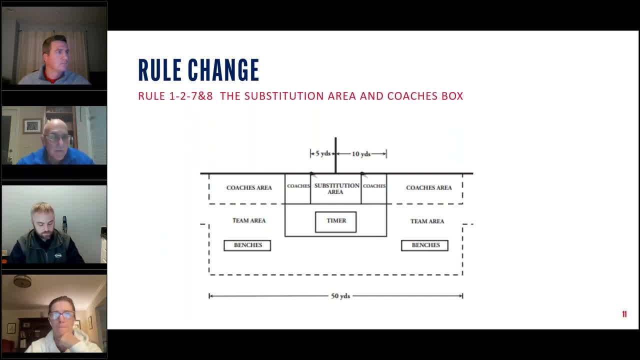 from to the five yards on each side of the midline, from the, so the 45 to the 45.. um, the thought process is is is a couple, couple ideas. we want to keep it the same as the ncaa, the college, and, and the next day we're going to be able to load them back into some of our situations. 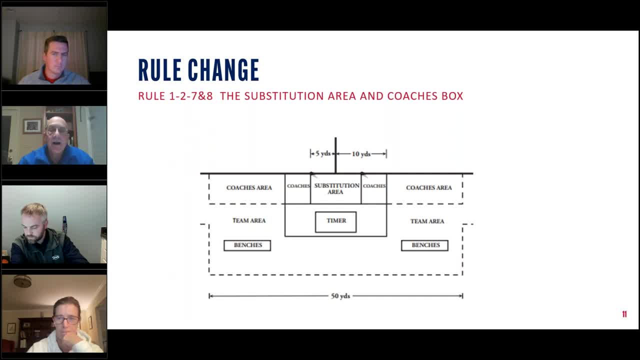 we're going to be able to get the. that's a good one, um, um, um, um, somewhat dangerous for officials who are in transition, transitioning that 20 yards and being in the way of substitutes coming in and out of the substitution area and creating a little bit of a safety issue for both players and and officials. and, uh, it was. 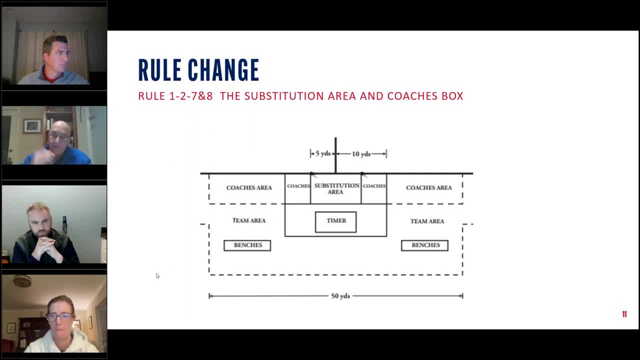 felt by a number of people that shrinking it back to five on each side and having that cone uh for us to to maneuver around uh makes it safer and easier for us to uh manage that that area. for old guys it's just back to back to what we did for years. for new guys, 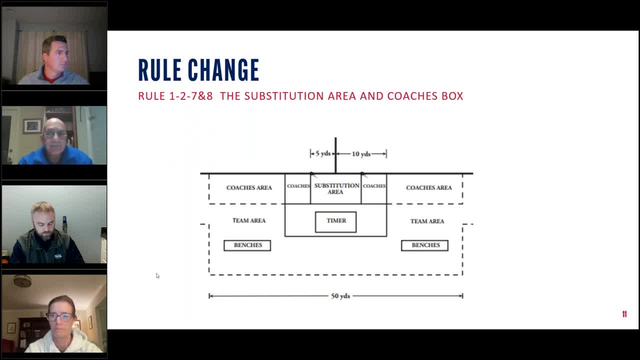 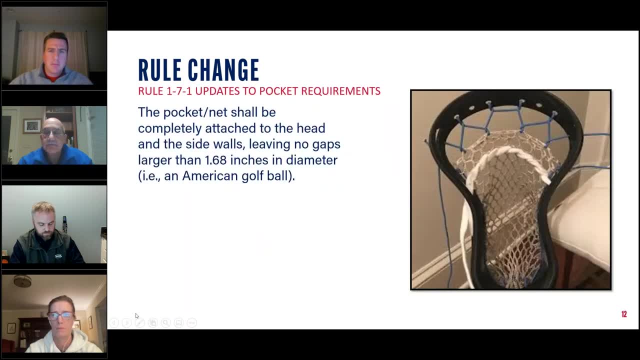 they'll see the shrinking and i don't think it it'll be that big of an issue. great, thank you, uh. next update to the pocket requirements: um, the pocket shall not be completely attached to the. the pocket shall be completely attached to the head and leave no gaps larger than a 1.68 inch in diameter- uh, the size of an american golf ball. um. 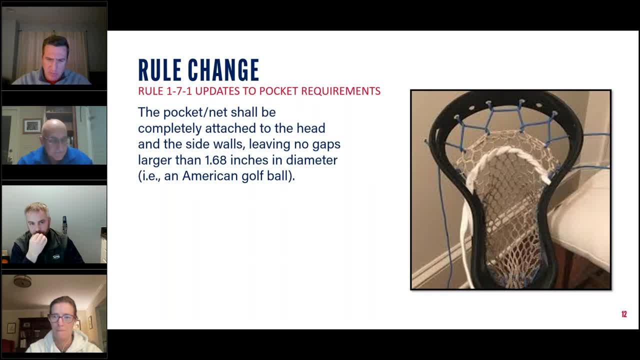 this might be a better question for james and uh and caitlyn, you kind of want to talk about, uh, what the discussions were at the committee and you know maybe where this came from and other rule sets, uh, and some of the success. can we go back to the box question? i'm sorry, i want. 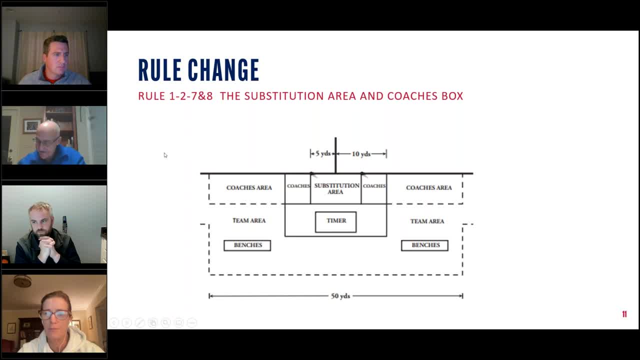 i'm all like one step behind you getting the questions in the box. um, i'll pause next time. my apologies, no, no, no, i put my hand up. i don't know if i have a hand thing. um, jim, are we clearing the box in transition again? that's a great question. um, we are not going at this point. our mechanic isn't to go back into the 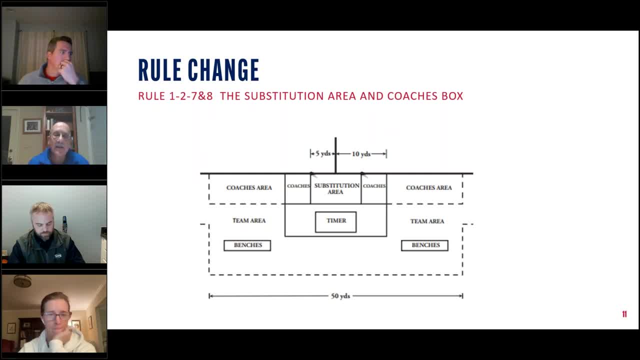 box and go down and clear everything. at this point, uh, that's something that can be discussed in, uh, in december and january on on what our mechanics are going to be, uh, but at this point it would be very, very similar to what we do now is is jog through it and if the trail, if there's a three-man. 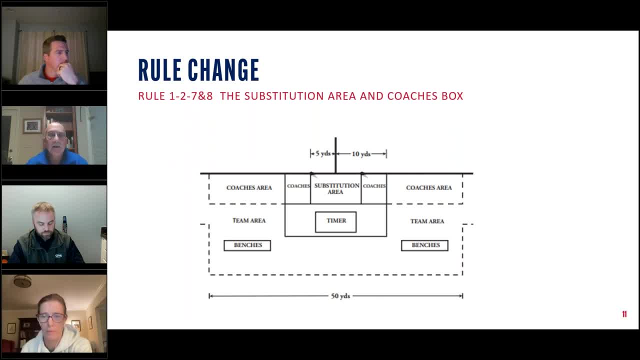 game. uh, the trail will come up and and and clear it and uh are in a two-man game, probably not. and then the follow-up question on the box: um, are two extra cones required to keep players away from the box? no, i, i think the cones, and i don't know if you can see my mouse cursor that typically. 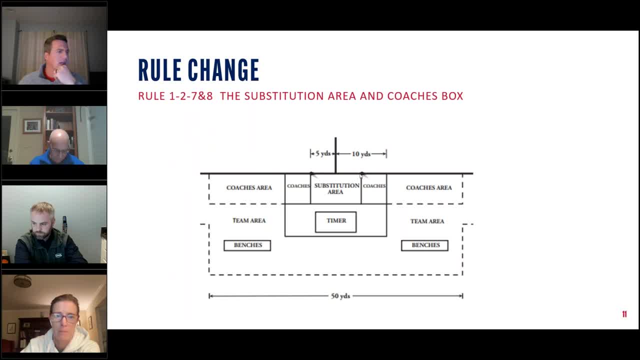 would be placed here at 10 yards. you're just moving them in um. there's not extra cones that is required. am i incorrect in that? no, i think that's correct. you're just putting, you're moving the cones from the 40 to the 45. right. 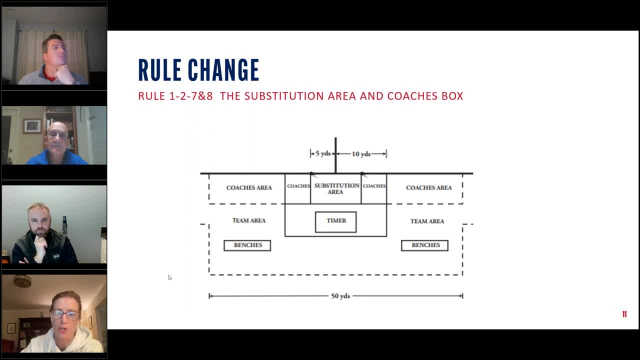 anything else? well, so they say, please, the coaches box is shown on the slide. yeah, the coaches area, uh. so the reason that, uh, i chose this image in particular here is, um, some fields might already be marked, meaning they came in and they had their turf uh, painted permanently with the substitution area. so what this is meant to show. 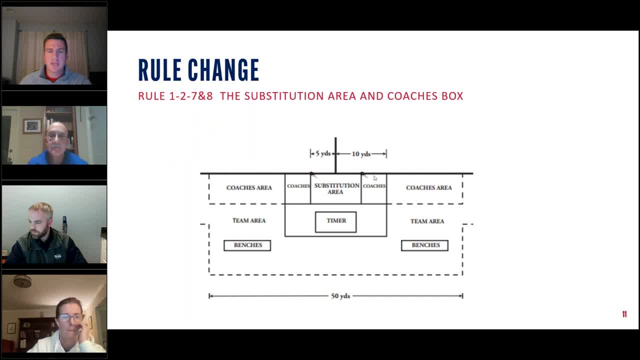 is. this was the typical uh coaches area previously and this was the typical substitution area, so all you would be doing is placing a cone here and here and then you put your cone in the middle of the here instead, and this additional area becomes part of the coaches area. that's all this is meant to. 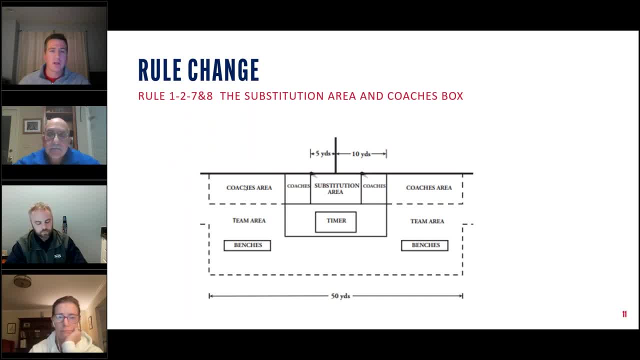 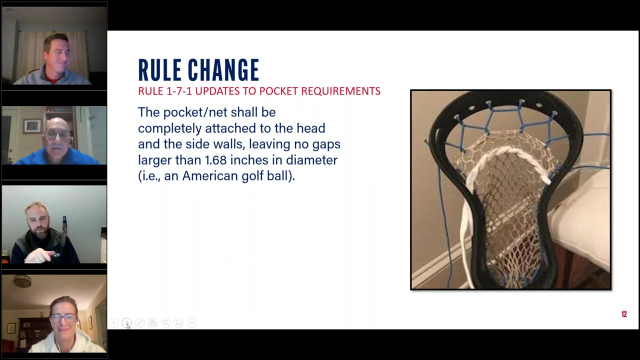 show um, because i know that that is going to come up and people are going to. you know, assume it's marked. what are we supposed to do? just place the two cones five yards off of uh off the line. that's great, thank you. do you want to cover this? yes, please, yeah. so what we've been starting to see as this is a um rule. 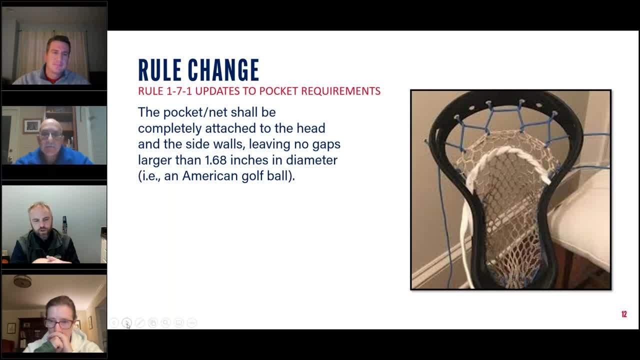 change that's happening before. we started seeing a lot of issues. we started seeing issues with alternative stringing techniques where they're leaving a gap at the top of the, at the top of the cross, where it passes the stick check, but then, once they put some pressure, apply. 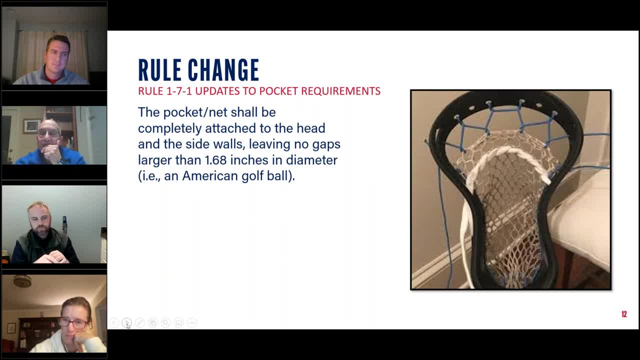 pressure, they can actually grab the ball with the alternative stringing technique. so by having the no gaps larger than 1.68 inches, it prevents that from happening. great, and and you'll see on that stick, the head of that stick, you'll see on that stringing. 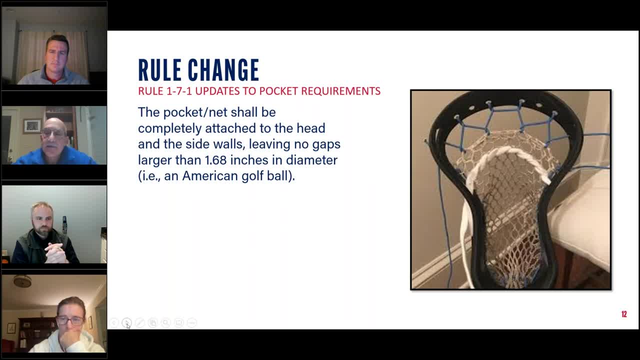 that he, they've left out the two lines, the two areas, what that's supposed to be strong and that if you read in the rule book, it says has to be completely attached. so those you look at the Buddhist rulebook, you see the bridge a little over the upper side and then that's what. 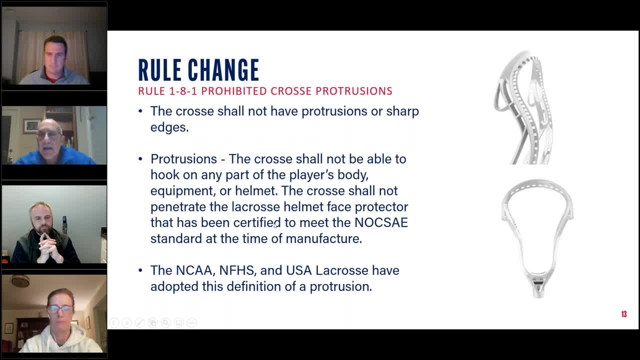 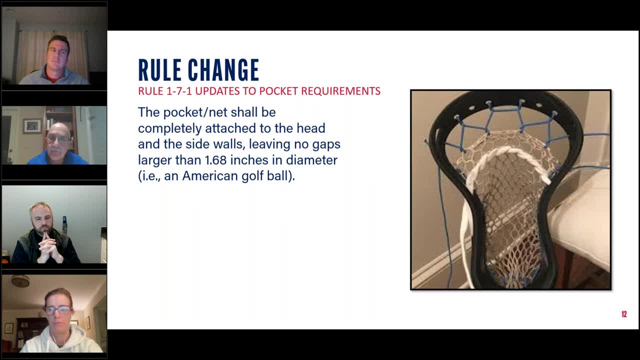 I'm going to leave aside, and the next seven, the remaining string. this will be on the poor to be at that stick, and and right there. that is in violation of the um, of the rule where it says it must be completely attached. so, um, that would be an illegal stick. yep, and for those that do, um, 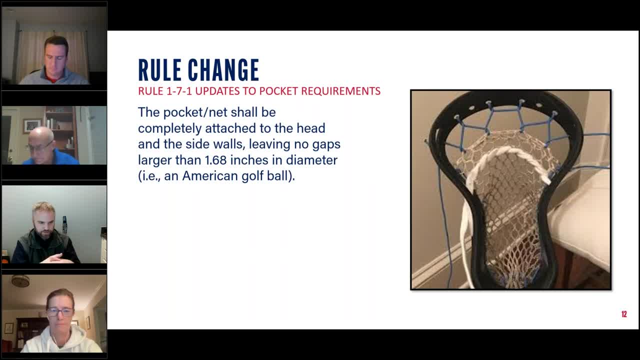 both girls and boys lacrosse. you'll notice that that 1.68 inch deal is in both rule books. as far as the gaps that are not allowed, right consistency. someone asked if you have to carry a golf ball. i do not think you need to carry it. 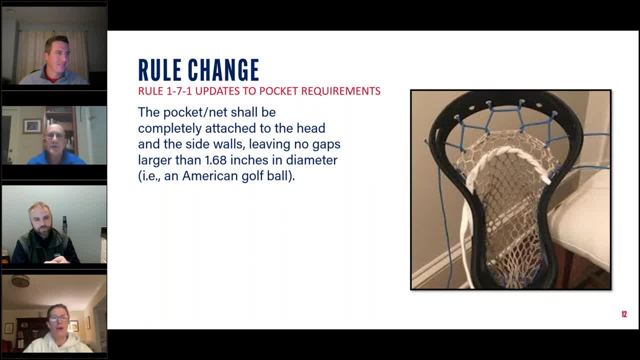 no, no, no, but we were trying to give a commonly understood size of something in order to make a. um. yeah, rick and i spoke about this, uh, this morning, and we're not putting anything else in our pockets, we're not carrying a utility belt, for, for all all the things that that are going to make this, this game, uh, more. 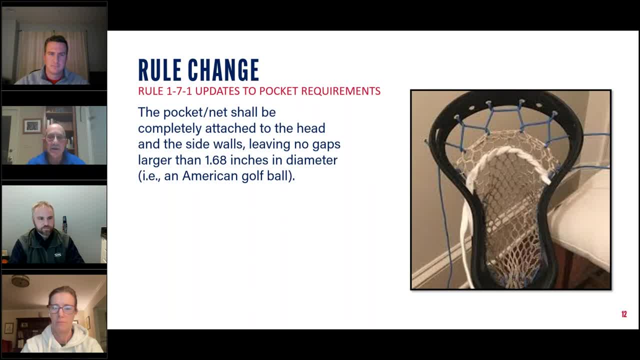 anguishing for for officials. just look that, if the stick has been altered- ie the one you're looking at right now, where he has restrung the top and omitted two holes- okay, he has altered that stick. it is illegal. okay, you don't have to stuff a golf ball through that to tell him that it's got to be. 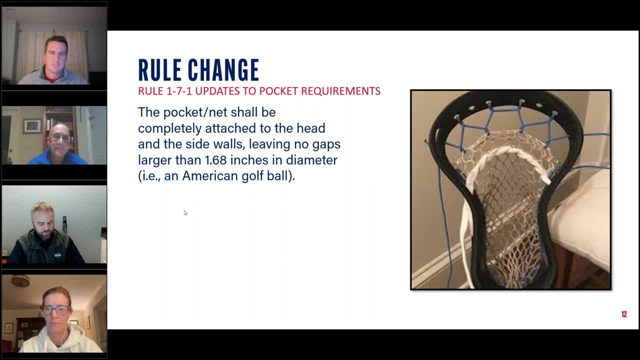 a golf ball. so if you have a golf ball right in there and we've got six holes of the same size, um, all the guys are shrimp and there's the end of the story. we're going to look at a golf ball and then figure out what we're going to put on the outside and what we're going to put on the inside. 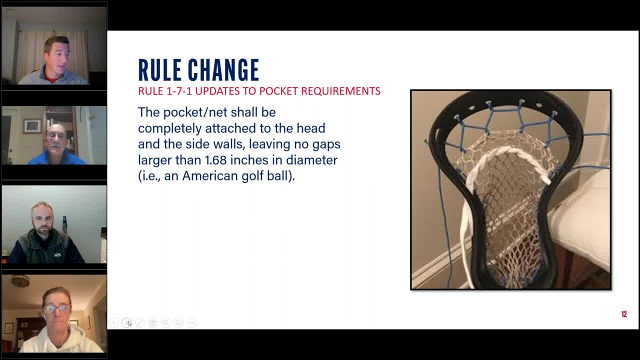 and that's going to be our golf ball instead of 4-2-3, right. so we're going to look at the front door, we're going to look at the outside, which is the cove, the wall, the middle section, the back, and it's going to be- um, it's going to be a little bit moreif you'll not be able to see it. 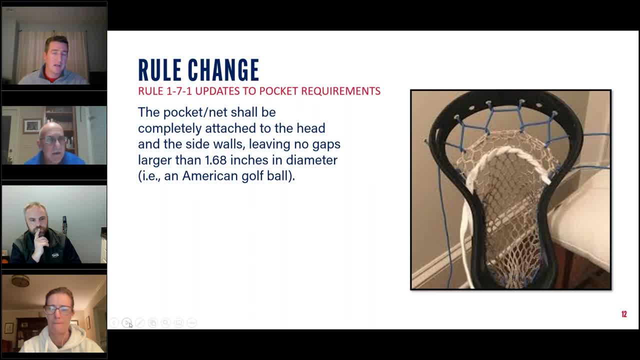 right now, but you'll get it there and with um, with all of that, you'll definitely be able to. at least is not an illegal stick. a broken cross is a no cross, so he's playing without a cross. so typically, i don't know if this question is: is, uh, getting ahead of ourselves because we're going? 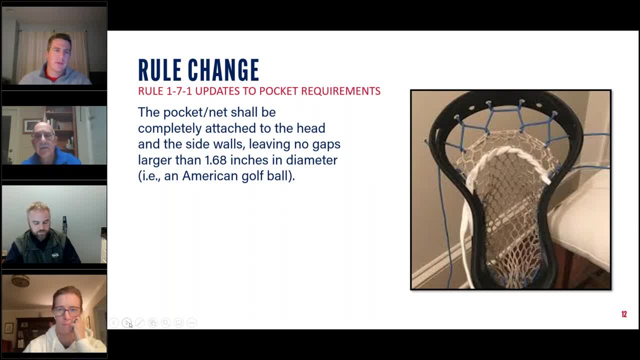 to be talking about, um, some issues, uh, that have changed our clarifications. with the goalie when they're out of the crease. but yeah, this is not a broken cross, this is just strung incorrectly. it's been altered. a broken cross is when the shaft or the head are broken so that they're 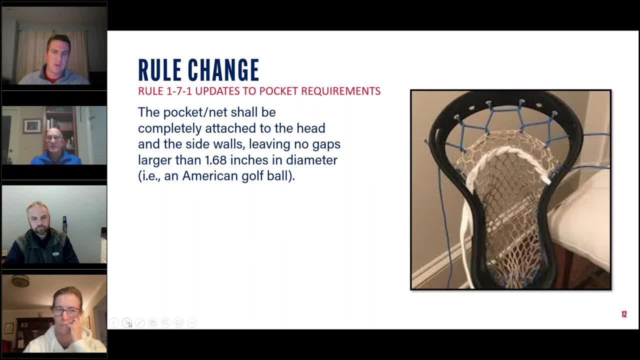 unplayable completely. that's that's when that would come into play, that it's a no cross. this is intentionally done, so a person just asked for clarification, um, that this would require the stick to be removed from the game in a three minute penalty. two minutes, one minute, very good. 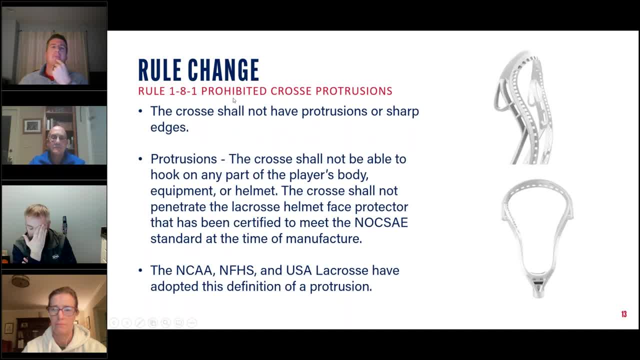 okay, uh, another rule change: um, prohibited cross protrusions. uh, it probably would just be best for caitlin and james- since you probably talk about this on a day, maybe a weekly or a daily basis- to kind of talk about, um, where we are and some of the consistency that, uh, that you've been trying to um. 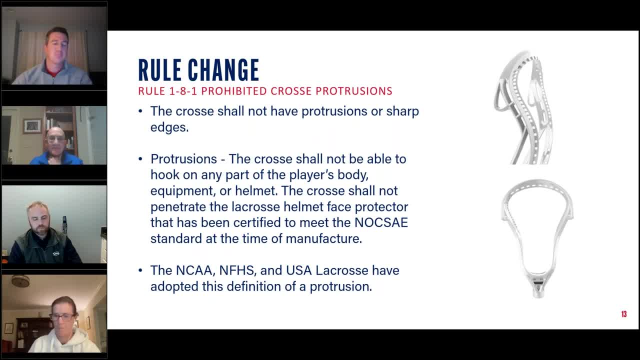 to bring to the world uh, with the ncaa. um, please, you know you want to do this, caitlin, or me to do it. i'll let you go first. thanks, all right. so we started seeing some new uh stick designs hitting the market and you'll see as uh, as noted on the screen, some of them have protrusions and we had 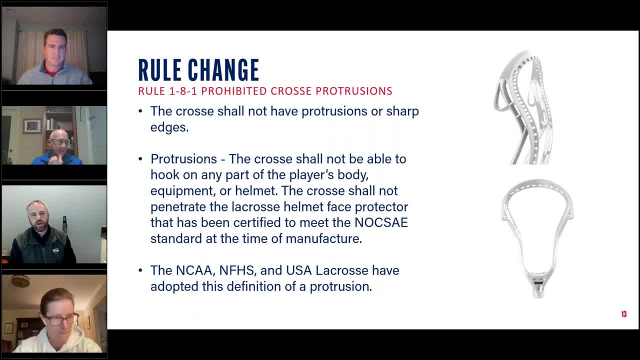 a big meeting with the manufacturers to talk about the safety issues that come with this. the protrusions on the particular sticks are easy to grab. the base pass. they're easy to grab the the shoulder pads and horse collar kids. uh, just very easy to make those kind of things. so we've 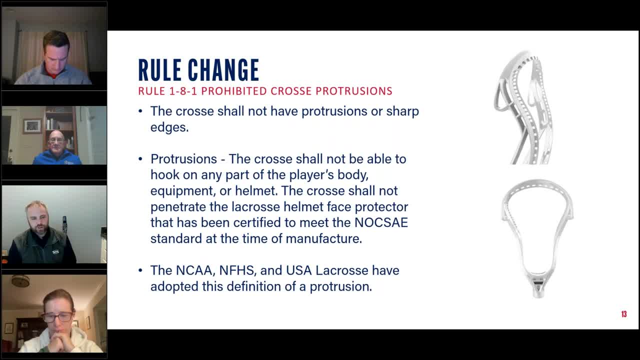 we sat down with everyone again with a good definition i think everyone's okay with, and we said: there's no protrusions or sharp edges allowed. and then the thing that i wanted to avoid is: i don't want anyone bringing a protractor onto the field. jim doesn't want golf balls, i don't want. 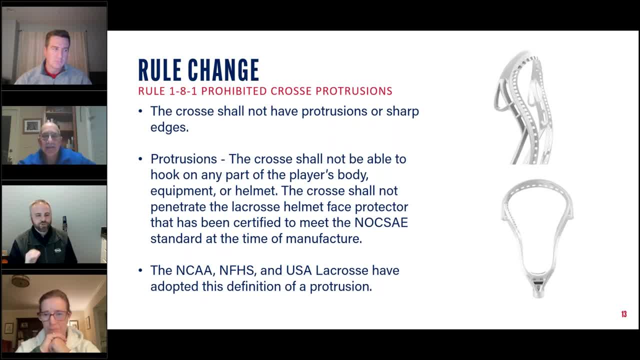 protractors right, so we're not going to measure these things out. so what a protrusion is is it's. the cross shall not be able to hook on any part of the player's body, equipment or helmet. the cross should not penetrate the lacrosse helmet face protector that has been certified to be the. 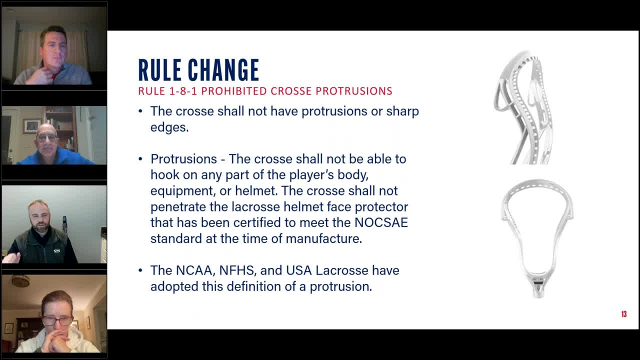 nazi standard at the time of manufacture. so basically, if this is able to hook on equipment, it's an illegal stick. we should catch most of these before they hit the field. so i'm not super concerned. but at the same time, just know that if a stick is grabbing onto equipment while you see it in the field, that would be an illegal. 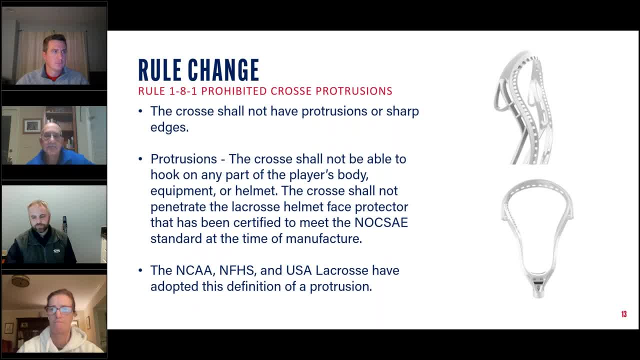 an illegal stick. caitlyn, what did i miss on there? i think you're good. yeah, i'll just add that this previous weekend i saw the ncaa rules presentation. so just to echo what, caitlyn and james, this is an ongoing conversation that the governing bodies are having with the stick manufacturers to. 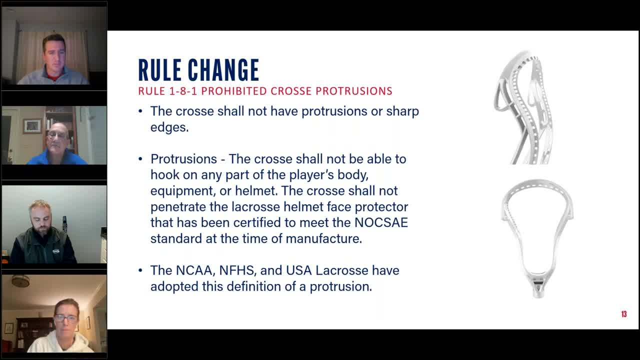 ensure that sticks are made safe and fair. so this isn't the last time this will be talked about, but this is the guidance that is at every level. uh, it is consistent among all the governing bodies. and add to that rick, i think, the thing that we've all discerned: the timing of the governing bodies. 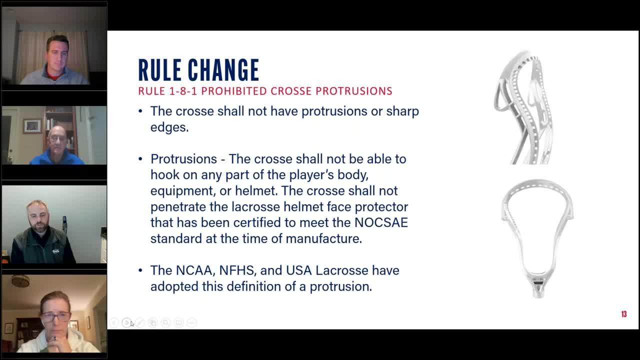 is player. safety is number one and if these stigma, if these stick uh designs are causing safety issues, we want to stop that before it becomes a widespread area, right, and that that will be up to the governing bodies and and knoxie to determine that level of stick. um, what we're concerned. 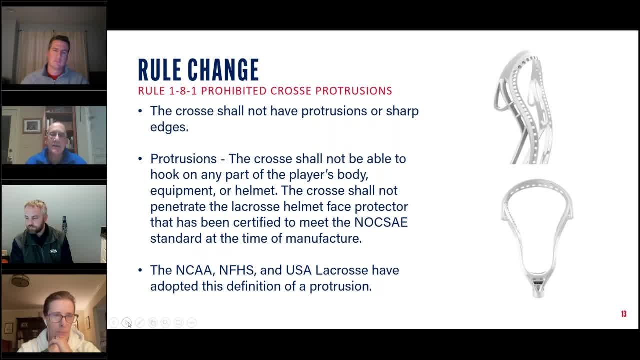 with on the field on tuesday is if a stick has been altered to to create a protrusion, we are not saying, we are not as officials on the field on tuesday saying, uh, the the rick lake, uh, shazam is illegal. okay, we're not going to do that, we're going to see just altered sticks. 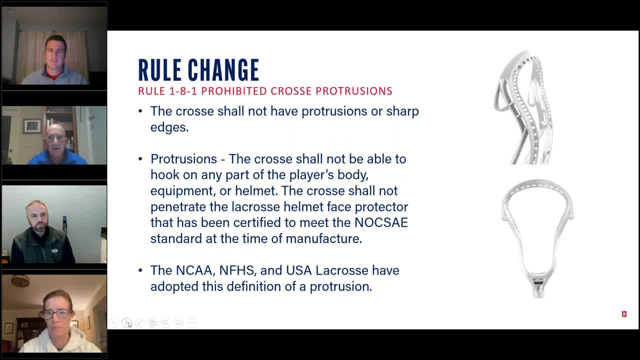 we are not ruling out certain manufacturers. that's not our job as officials, that's the job of the boards: the federation, usa, lacrosse, moxie and the stick manufacturers. so we're only looking for sticks that an individual has altered, much like the stringy and the 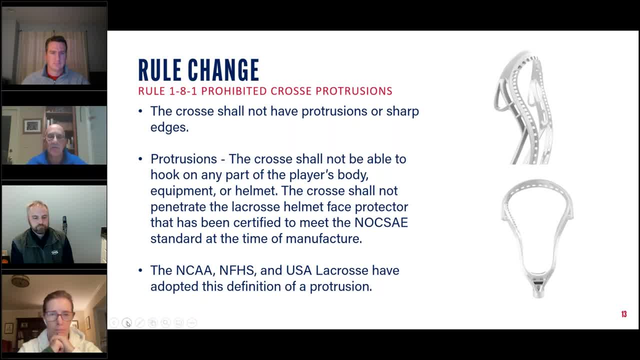 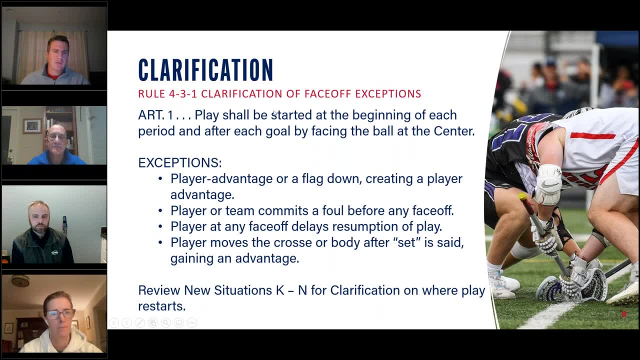 slide to gain an advantage, not not a manufacturer's stick. okay, uh, the next one. um, i think this is one that was maybe not in, uh, the pressures that came out, but it was something that was an important clarification that came, uh, for face-offs. so, jim, do you want to talk about, um, you know possibly why this rule came about, and maybe some. 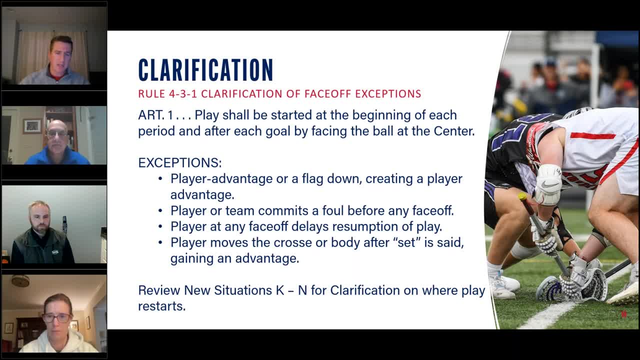 of the confusion that was occurring due to fouls that were occurring immediately after a face-off. uh, yeah, uh, essentially, if you've got a, a face-off violation, uh, you're starting everything, uh, in the offensive half of the field and with a whistle and and a 10 count. 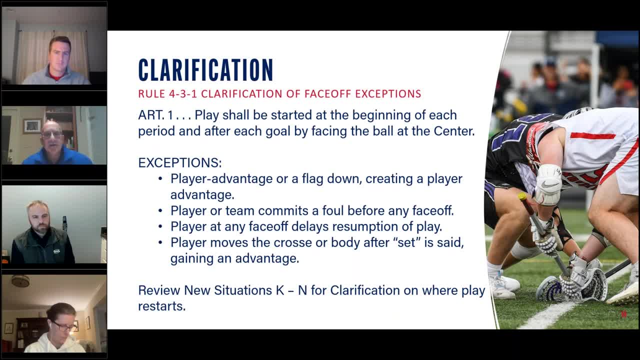 the only time you are not doing that is if a team has three men or more in the penalty box, and if you're not doing that, you could take a defensive player up to do the face-off. and now, prior to that face-off, the other team violates. so now that 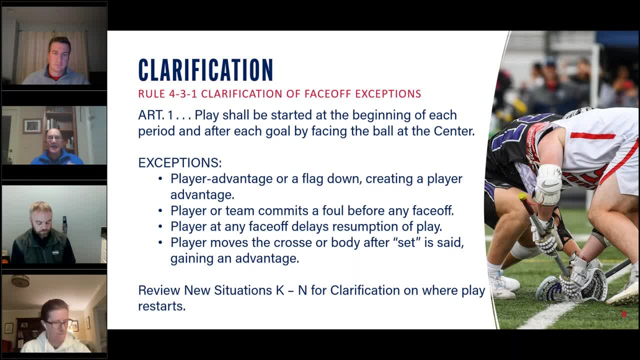 defensive player who's doing the face-off must start the ball. he can't start in the offense because they need the offsides. he can't give it to an attackman because they're not released from the below the restraining line until the whistle starting play. that player has to start in the defensive half of the field and he has then 20 seconds. 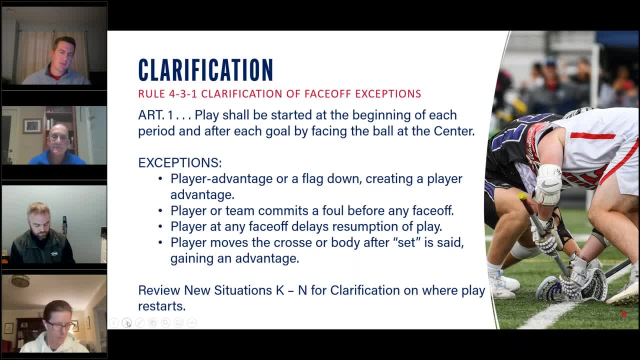 to clear the ball. yeah, there's a a series of new, um, new situations that are in the rule books. that are situations came through and jim just very briefly summarized all of them. we'd encourage everyone to go and read them, uh, before the start of the season, and then make sure that you're. 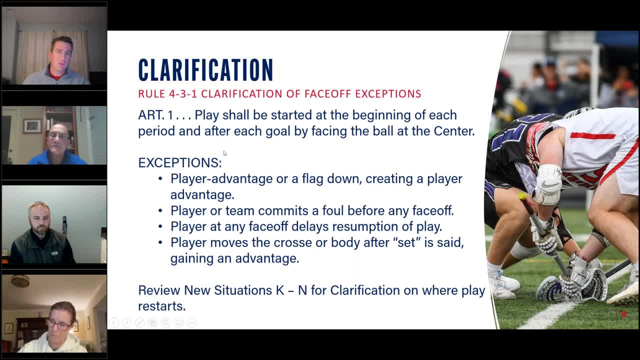 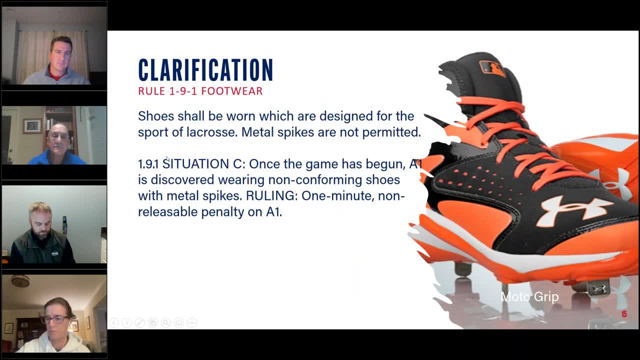 looking at, uh, all of the language that's been updated within uh the face-off exceptions. clarifications on footwear: uh, how many pages of the book were taken out to uh clarify what? what's what shoes can be worn in lacrosse games? james, three pages, three pages for saving trees, um. 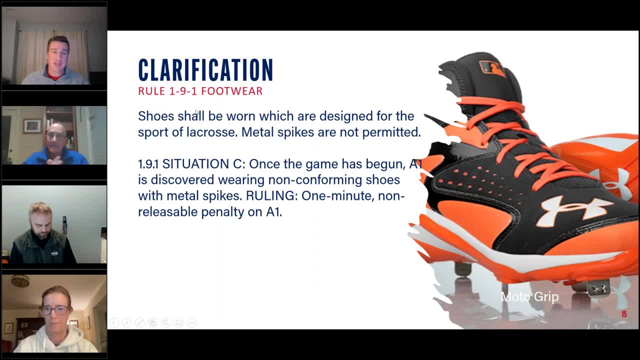 i could just talk about this one very briefly, since it's not really in depth. uh, shoes have to be: uh, for lacrosse. you can't wear metal spikes. you can't wear metal spikes. you can't wear metal spikes um within the shoes. um, and again here, just for clarification. 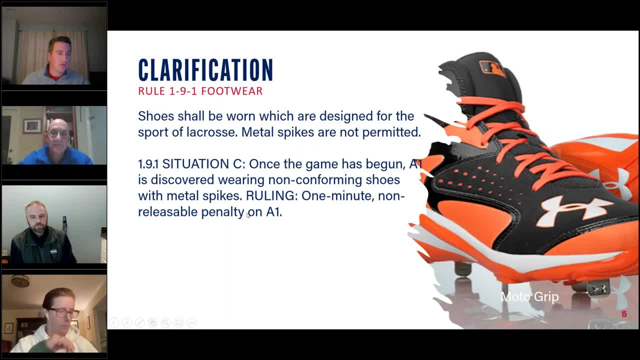 uh, it's a one minute penalty, uh, non-releasable if a player is wearing shoes that do not conform to uh to the rules. caitlyn, yes, oh, i thought you had a comment there. i'm sorry i saw something. no, no, it says metal tip studs on grass fields. this is a. is the question uh. 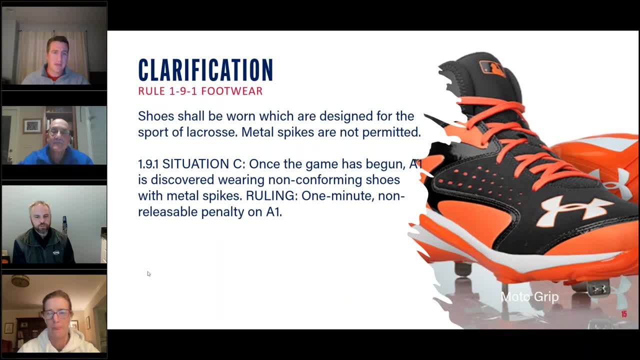 if it has metal on it, it's a metal spike and it is illegal. metal is metal, you got it. metal is so 1970s, um and then uh. the um follow-up question is: once the player serves, the penalty are: how do they get back on the field if they still have metal spikes? 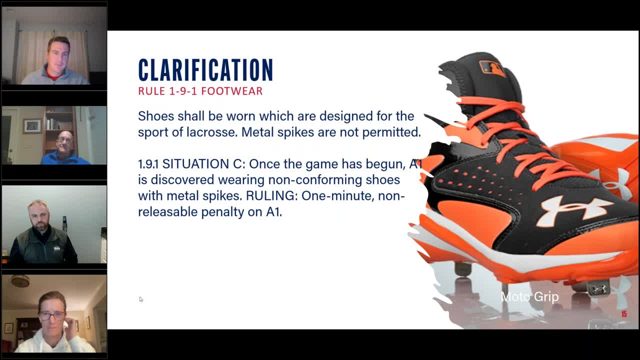 to come on the field, you have to be properly equipped. so, um, if they were to come back into a game and found to have illegal equipment again, they're going to get another penalty. thank you all. good, this is a huge clarification. it's easy, it's a huge update that makes it a lot easier. 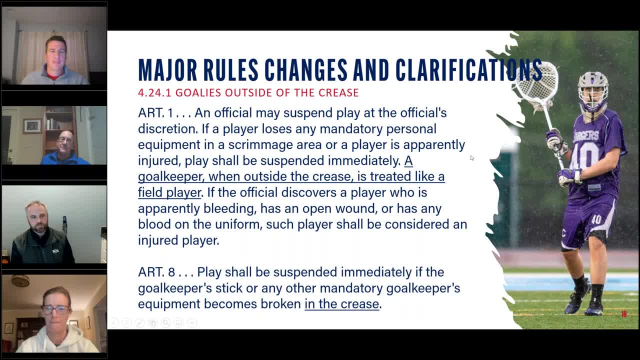 for everybody. yeah, it's something that's been a pretty much non-issue for a while and, at least in my area, wherever i've officiated, i haven't come across metal spikes in in years and years for a while. so i think it's something that's been a great way for us to try to find solutions. 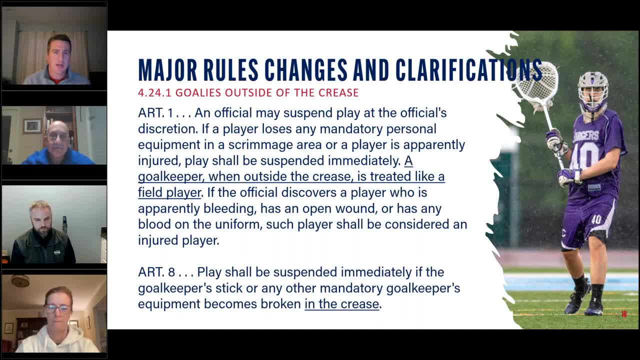 to sort of get that down to the ground and kind of go back to what you mentioned with the, the, the. the thing that we're trying to do is to kind of new the new rules, um, and i think it's going to be a little bit different for us as we get into the future. but i'd like to hear from you. 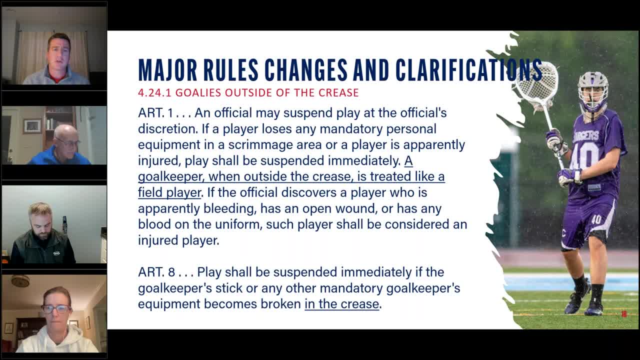 about some of those, um, new rules that you've been working on. i'm going to go ahead and give you a little bit of a brief summary of what's been going on in the field, um, and then we'll go into some of the other things we've been working on in the field. so i'd like to get your thoughts on that. 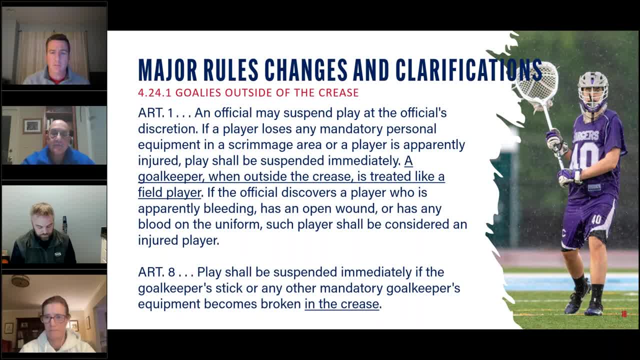 players, uh players, suspended immediately if the goalies, uh stick or other mandatory uh equipment becomes broken in the crease and that's underlined specifically. so, jim, do you kind of want to talk about that, maybe working from your crease outwards toward the rest of the field to talk about? 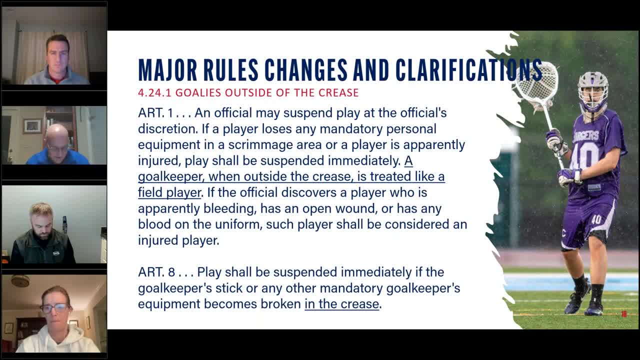 um, you know what this rule change means? uh, yeah, um, and and first, before everybody starts typing in a lot of things, we are aware that in three other areas of the rulebook it says that it that must have a fully equipped goalie on the field at all times, and we're going to try to. 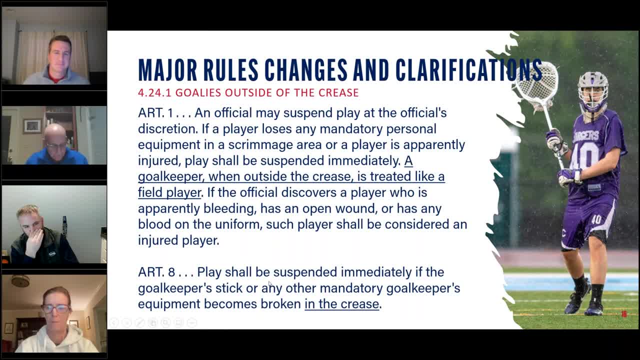 address that also. um, and we are aware of that and we've been talking about this since since august. um, but goalie in the crease has to have all his equipment, without question you. If he loses any piece of equipment in the crease, immediate whistle. 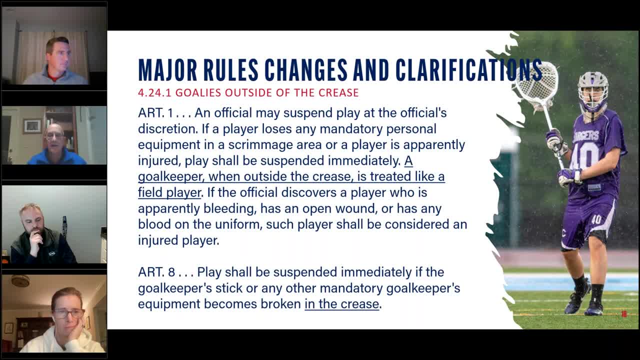 Immediate whistle making sure player safety. If the ball is in the crease, he gets the ball. If the ball is loose outside the crease, it's AP Whoever has possession. if there's possession on the whistle maintains possession. 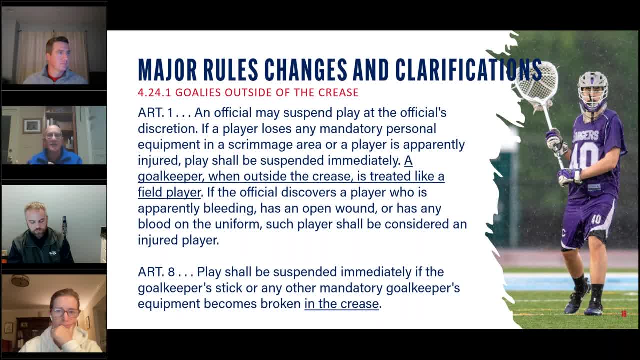 But the player safety, goalie safety, can't lose anything in the crease, can't be in the crease without all his equipment. Once he leaves the crease, it has been determined that we should treat him like a field player, And that's the wording: is: treated like a field player. 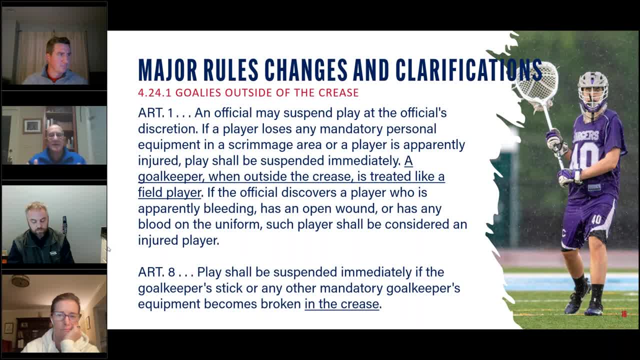 So that if he is playing, if he has the ball in his stick and he's clearing and he loses his glove, what would we do if that was a field player, not the goalie, and he had the ball? We'd blow the whistle, he'd put his glove on. 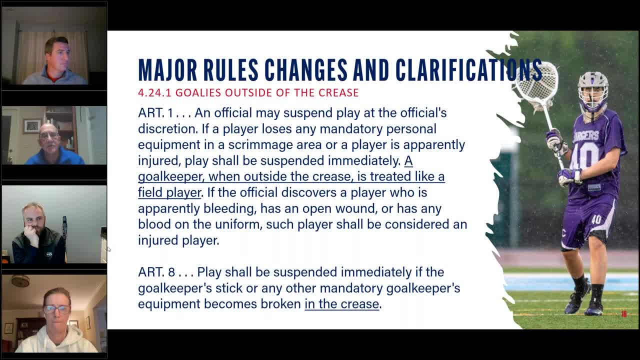 and we'd continue playing. okay, He's treated in that situation If he loses his throat protector. he's a field player who had possession. he keeps possession, he keeps going. He goes out of the crease now and he loses the ball. 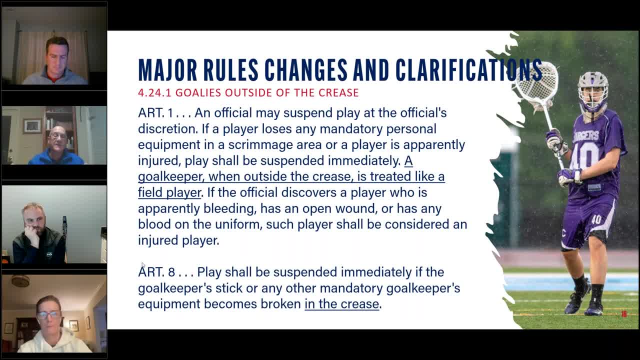 and he's playing a loose ball. Here we have a bit of an issue and situation that we have to address. He now checks a player's stick, trying to prevent him from picking up a loose ball, and his stick breaks. What do we do? 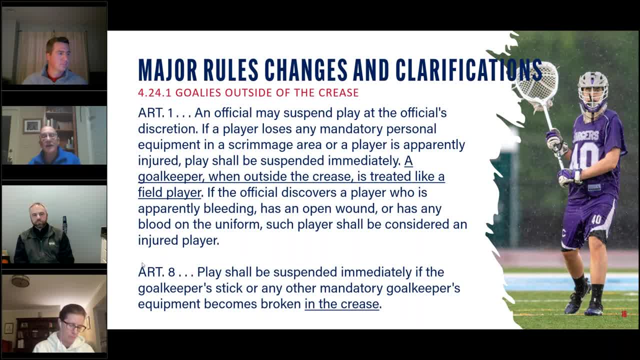 Well, again in the rule book, he's a goalie that must have all the proper equipment, yet he's out of the crease, so we have some contradictions. But if the ball is loose and he is in the scrimmage area, 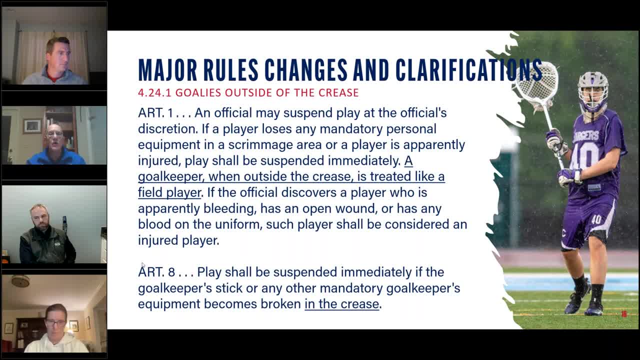 what would you do if it was just a midfielder who broke his stick and was in the scrimmage area? Would you call a play on You? could? Would you blow the whistle if he's in the area playing without a stick? If it's just the fact, 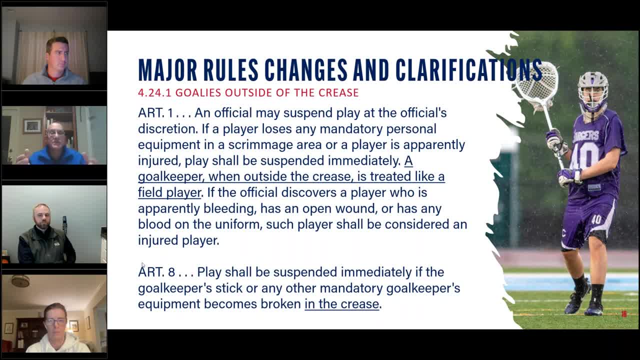 that his body is in the way of other people. blow the whistle. illegal procedure playing. The director has to go to court procedure playing without a stick of a team ball. this is how you would treat the goalie in this situation. if he's in the area and he's involved and he's interfering, blow the whistle, give the. 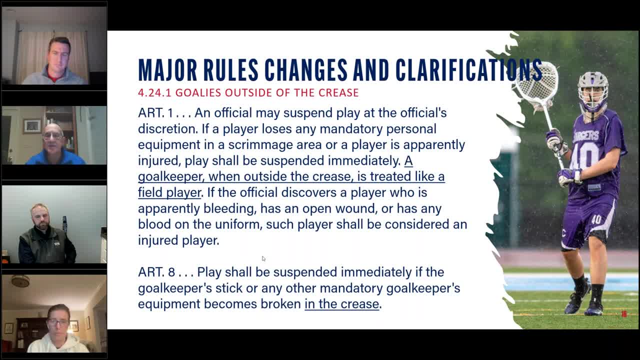 ball to the other team. now we have this situation. do we have a quick restart? now we have a dead ball, we have a goalie without equipment. it's determined that we're going to allow the goalie to get a stick, get his equipment and get back. get back in the crease, because we need a prop, a properly equipped goalie in the crease. 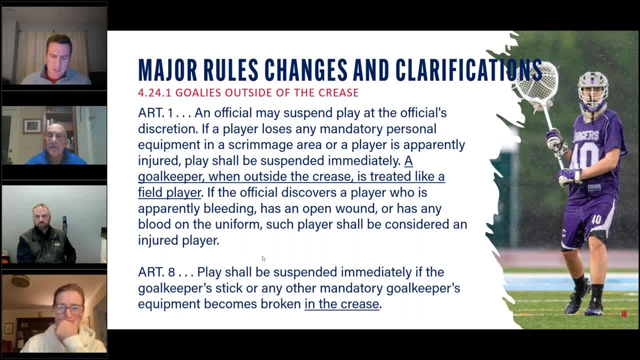 right and and this, uh. this builds off of a rule change that i think was made in previous years, where there was some, um, i guess, confusion about what happens if, sort of, we have a scoring play, which is eminent, uh, if someone's in the, um, the scrimmage. 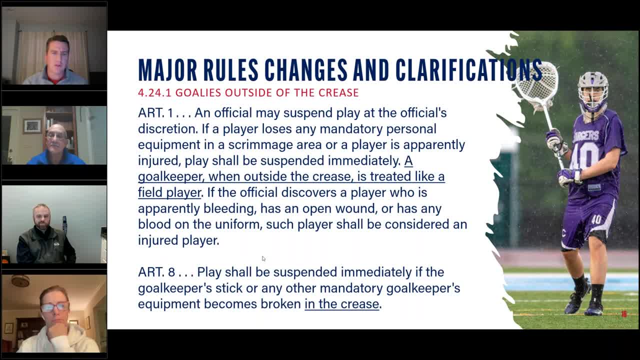 incident and we have a scoring play which is imminent and if someone's in the um, the scrimmage incident, and we have a scoring play which is imminent and if someone's in the um the scrimmage area, and i think the clarification is really looking to say that the goalie needs to be. 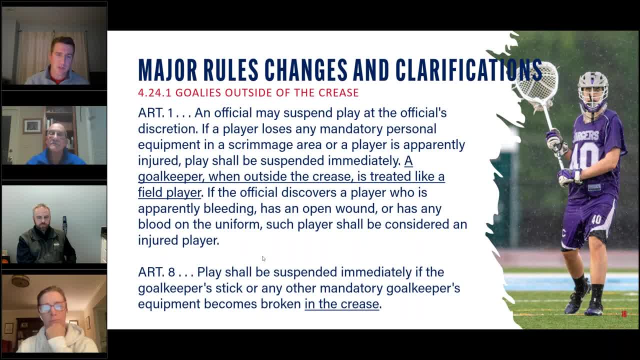 treated like everybody else, probably when they're outside of the scrimmage area and outside of the crease. um, you know meaning that, the way the rule book states it right now, if the attacking team has possession of the ball in the scrimmage area and someone from either team loses a piece of 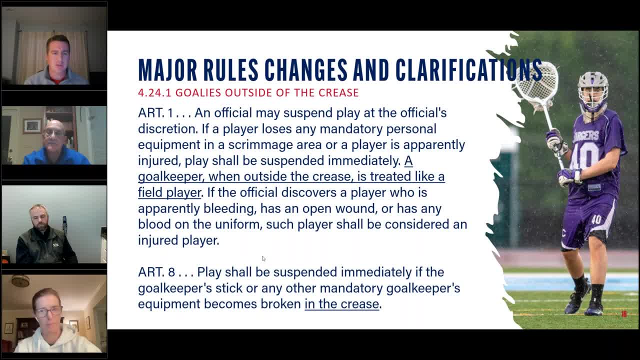 equipment, um, and it's not done, you know, intentionally so that they can kill. the play plays to be stopped immediately so they can get that piece of safety equipment on. uh, so that's where they're the only offense and defense. i think what this was looking to do is talk about um. 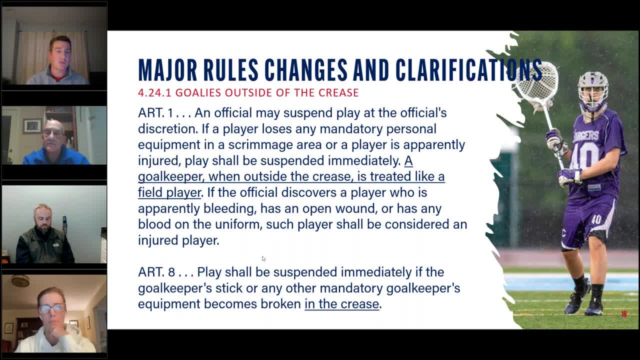 goalies. we typically talk about how they're special, where they have special privileges within the crease. they lose those privileges when they go outside of it, uh, and further outside the scrimmage area. so, um, you know, as jim had mentioned, uh, goalies are treated just like everyone else. 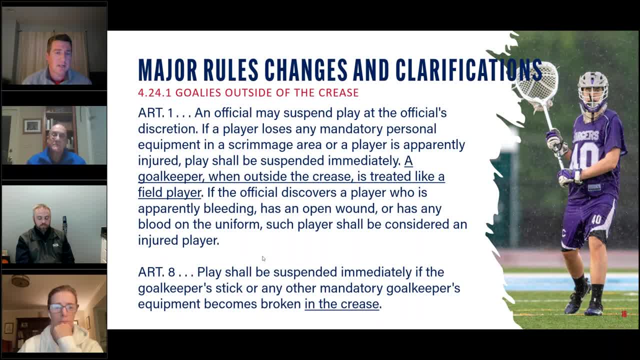 when they're outside of the scrimmage area and if something were to happen to their equipment, um, you know, and all the different instances in there. so, yeah, and that goes to that, the third scenario of of now, the, the, the offensive player has the ball in his stick and the goalie checks. 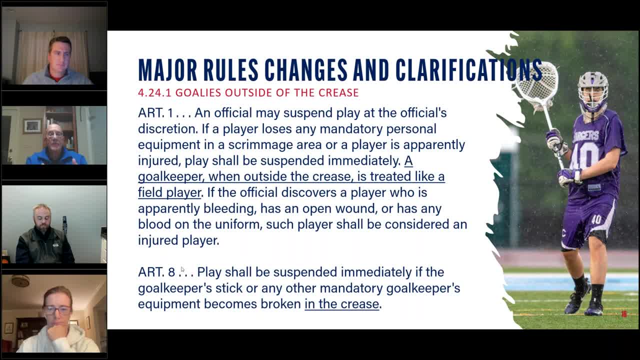 breaks his stick, okay, um, what we don't want to do is kill the play and kill the scoring play for the offense. and then that was the, i think, the major intent of of this change: to allow the offense to continue their offense when they have possession and the goalie breaks his stick or loses the glove, so on. uh and so. 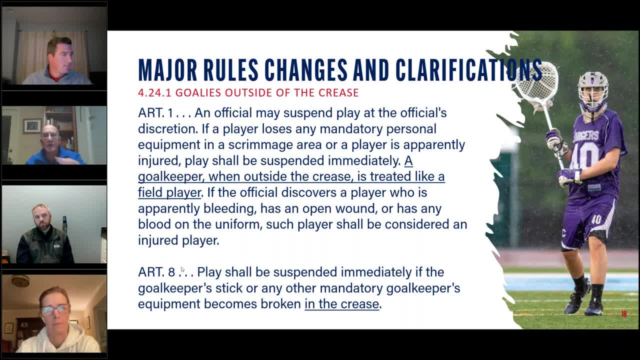 forth, loses, you know, loses a piece of equipment, so they want to continue. allow the offense as long as the, the, the safety of the players is is is not endangered. so if the goalie checks, braces dick. the of the middie. offensive attackman, offensive middie. 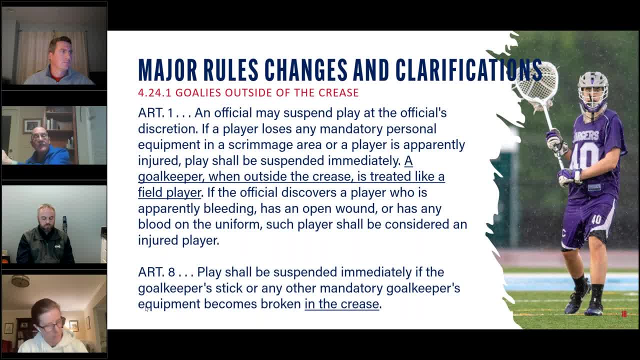 has possession and continues moving away from the goalie with the broken stick much like any other player. we allow the play, continue to give them, for them not to lose that advantage. Right and Jim, let me interject with a couple of questions too. 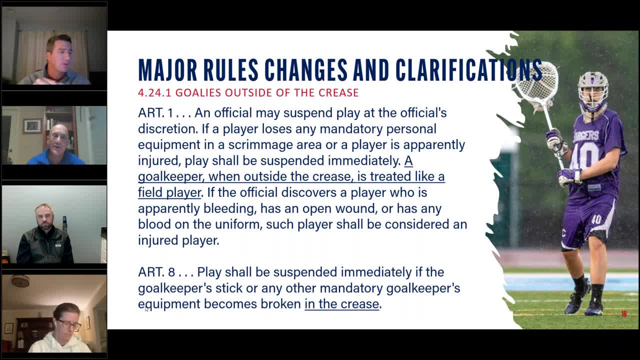 This had come before and I know we have some questions coming in, but I think we're probably gonna answer a lot of them. Somebody wrote in an excellent question: If a goalkeeper breaks his stick competing for a ground ball outside of the crease? 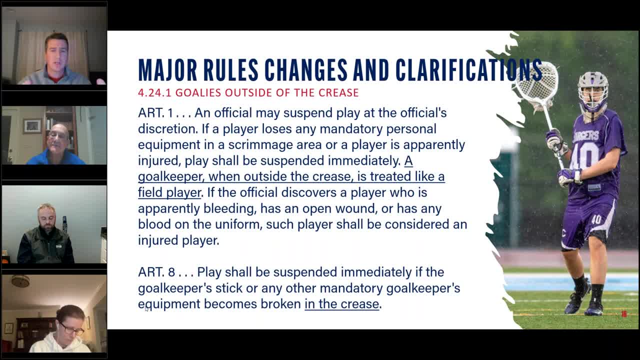 how is possession awarded? So for this, let's just assume that we're in the scrimmage area, the goalie is competing for a ground ball, loses a piece of his mandatory equipment, the ball is loose. how is possession awarded? Okay, you wanna answer that, or you wanna? 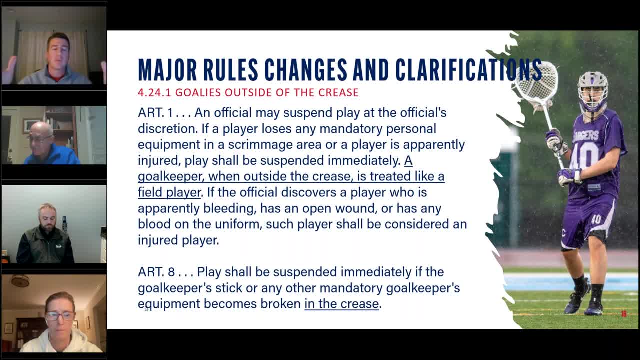 Yeah, the answer would be that's gonna go to AP, because if we have a piece of lost or broken equipment, the ball is loose in the scrimmage area, we go to AP, And if I'm wrong about that I apologize. That's in the old rule book. 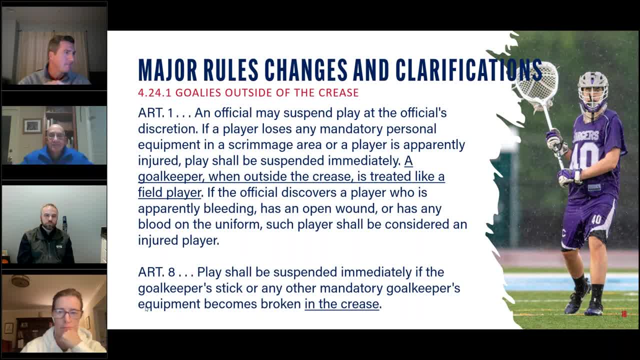 it's, yeah, the AP. we just don't. we have to kill the play the ball's loose AP. Now, Jim, if when a stick becomes broken and the defense has gained possession prior to stoppage and the ball's in the scrimmage area, 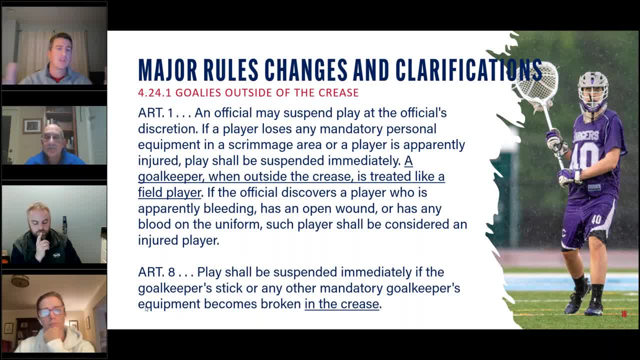 play should be stopped. Where should the play be restarted after we either get the equipment back on the player and the field's ready to play? where should the defense restart with the ball? The defense by rule can start anywhere in the defensive half of the field. 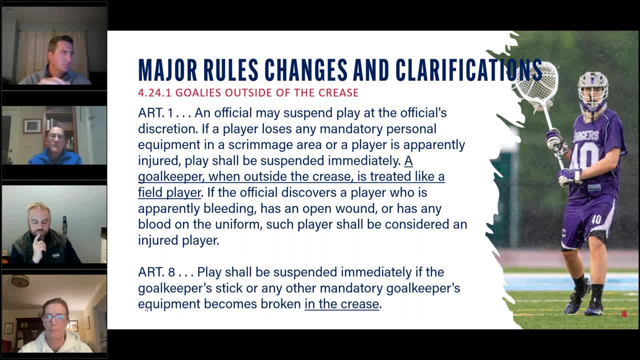 They don't have to take it out of the box, They don't have to move it anywhere. We- just we- can restart the defensive play at the spot again with people five yards around. Correct, Now let's take that situation. 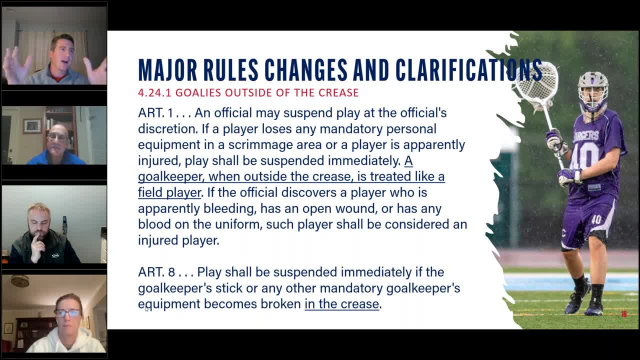 And as a stick breaks in the scrimmage area, a player on the offense gains possession of the ball prior to the stoppage occurring. Let's say that they were right in front of the goal. Where is play gonna restart? by rule, Okay, if we kill it and they haven't taken a shot. 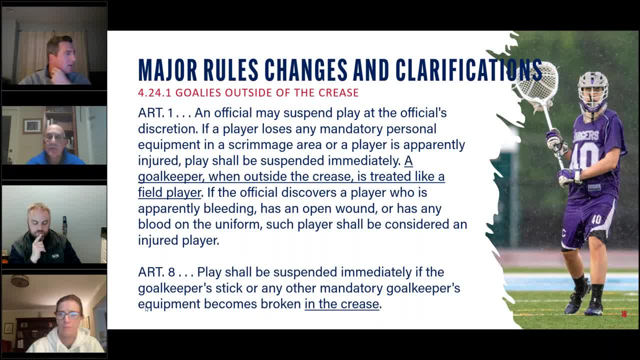 it's gonna go out in the alley, Exactly okay. So that was one of the questions that came in, But, Kaitlin, do you wanna go ahead and ask some of the questions that have been coming in from the audience? So two questions around, potentially what happens. 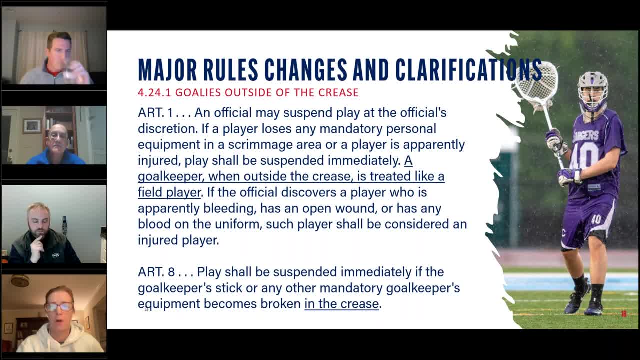 if the goalie purposely drops their glove or their cross Purposely? well, now you have a conduct or an unsportsmanlike. Okay, next one: What if the goalie's out of the crease and loses his throat guard? He then runs back into the crease without the throat guard. 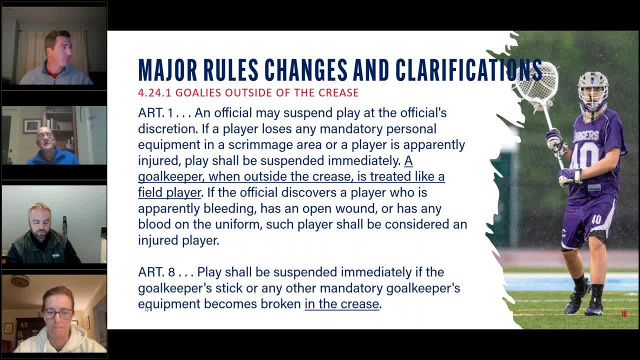 Do we stop play? Yes, and this is the conundrum we have with this rule. Yes, if the goalie loses any piece of equipment and starts heading towards the crease, kill the play. If it's a loose ball, kill the play. 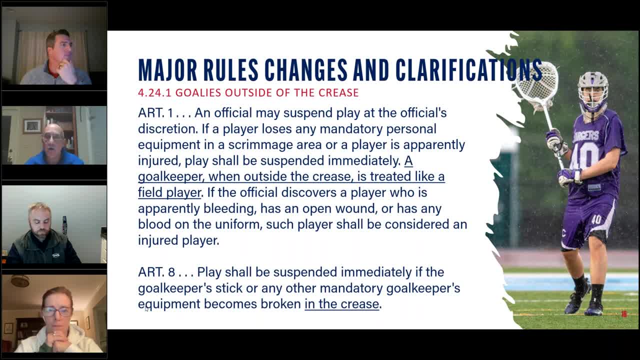 If he's behind the attackman, who is the goalie? who's got an open shot? let the attackman get the open shot, But if he's heading toward the crease- and he's going to be between the ball and the crease- 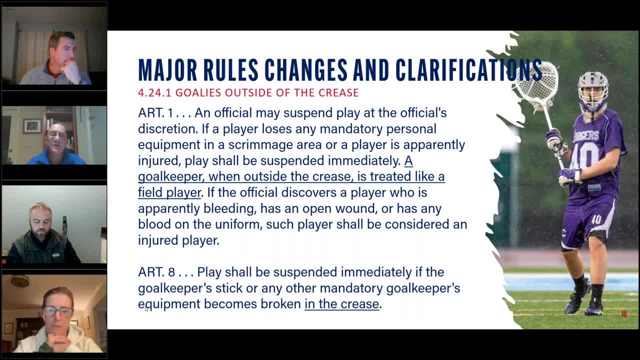 you gotta kill the play, And if it's a loose ball, it's going to be illegal procedure. offense ball. If the offense has the ball, it's going to be illegal procedure. flagged down 30 seconds, Which opens up a bigger can of worms. 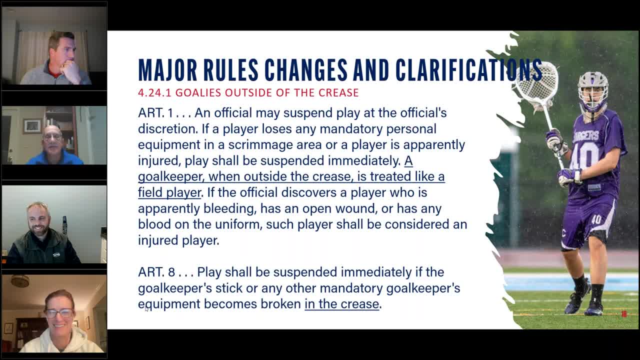 And I can see hear everybody typing in Mac those things, And just as a reminder too, that's on the first possession. If it happens again subsequently that turns into a one minute unsportsmanlike foul And it remains that way. 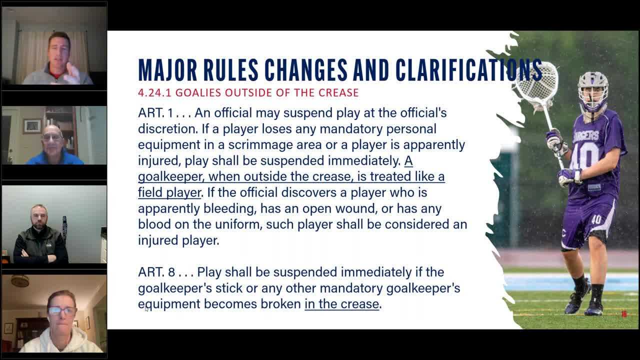 And the player that caused the injury or not the injury? excuse me, the player that caused the foul is the one that serves the penalty. Correct, Correct. Any other questions? Katelyn Got through that. Yep, we're good right now. 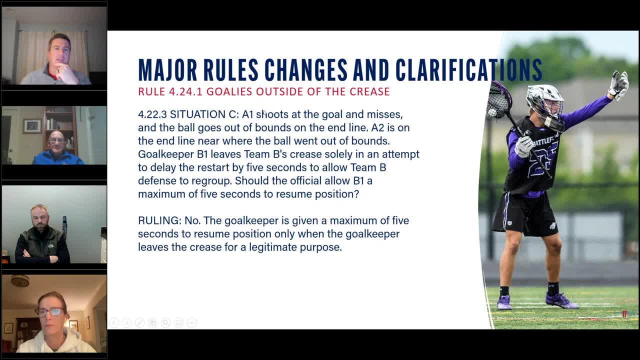 Good to know. Okay, Moving on goalies outside of the crease. Okay, So this, Jim, this situation deals with a goalie and the allotted time that they have to get back into their crease. Can you sort of talk about what we discussed earlier today? 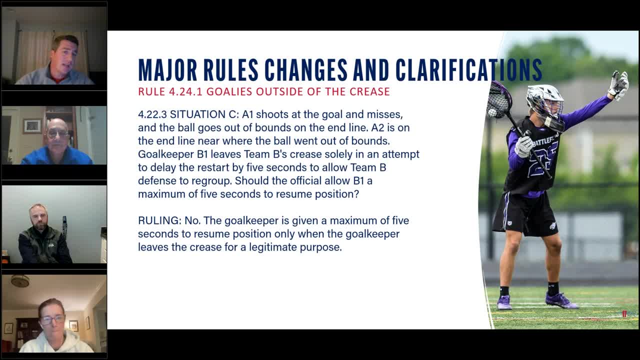 about, you know, the five second rule. do they get up to five seconds? Do they get five seconds? And what should officials be doing to ensure that this rule is used properly and that goalies aren't, you know, sort of using what they think is an attempt? 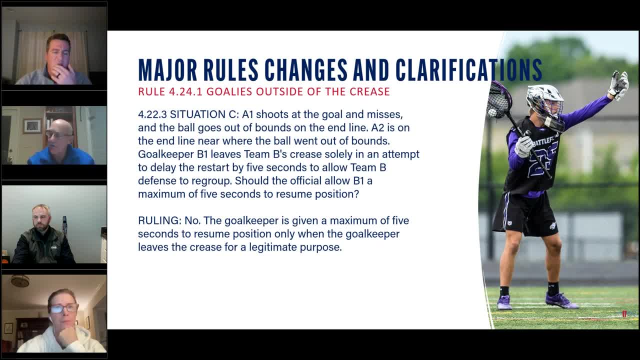 to sort of delay the game. Yeah, the goalies always have a chance, always have up to five seconds to get back into the crease upon leaving the crease and a dead ball whistle if they have been active in pursuing a loose ball or clearing the ball situation. 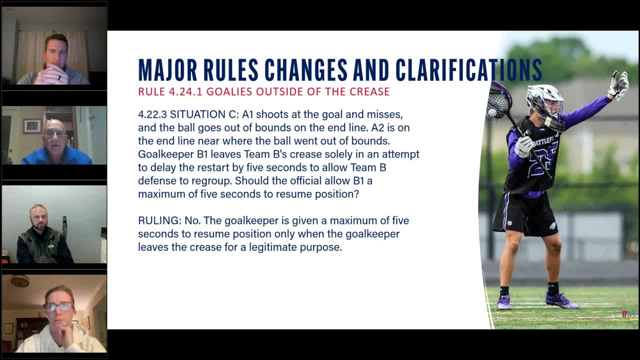 I guess we've had some issues or incidences where goalies have left the crease to just delay the game and allow middies to substitute, or a different defenseman to cover the attack with the ball, so on and so forth, And this is why this has been put in. 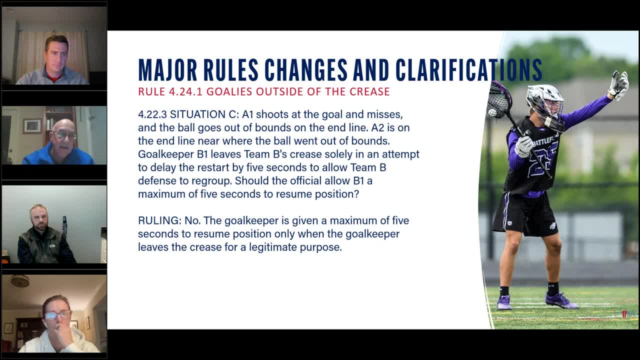 And you don't say: well, you're only going to get two seconds this time because of it. If he is deliberately delaying the game by randomly leaving the crease to then demand five seconds to get back in, we use our managerial skills and have a talk with him and his coach that he's delaying the game. 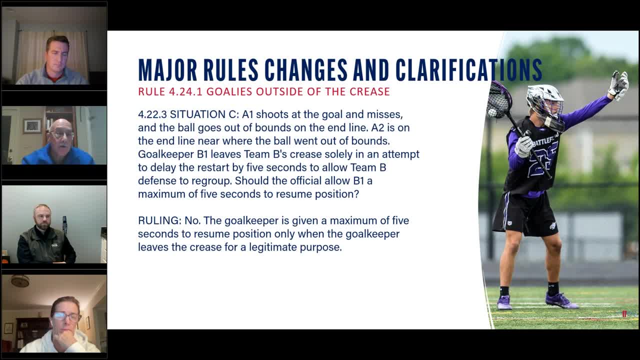 And that could be a conduct foul or a legal procedure. delay a game and move on from that, But we're not going to say to the goalie: well, because of that, you're only getting two seconds next time. No, we'll give him the proper amount, up to five seconds, to chase the ball to the end line. 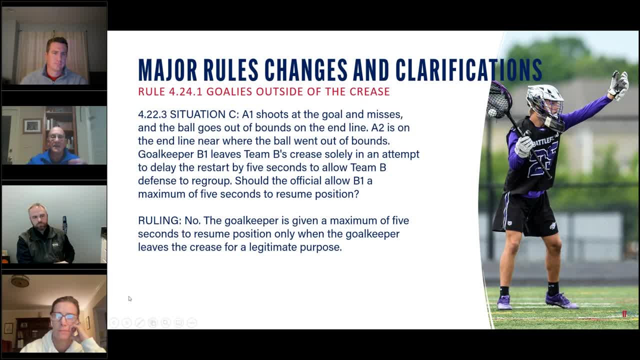 He doesn't get it, He heads back. You give him the count, He gets in, We're good. He clears the ball, He loses it, or whatever happens, The ball goes out of bounds. He gets his five to go back. 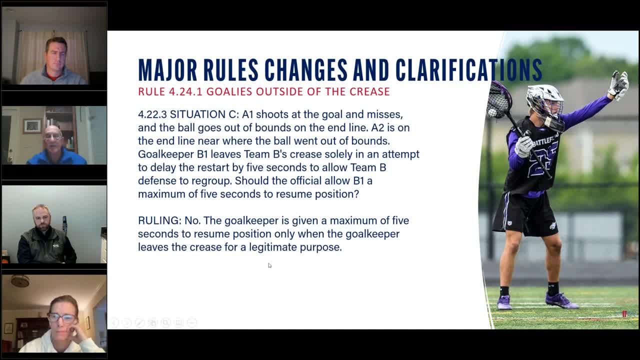 All right, And we don't say: well, you're only getting two this time. If he gets there in three seconds, start it in three seconds. You know, don't just keep waving your five seconds, because that's what the rule book says. 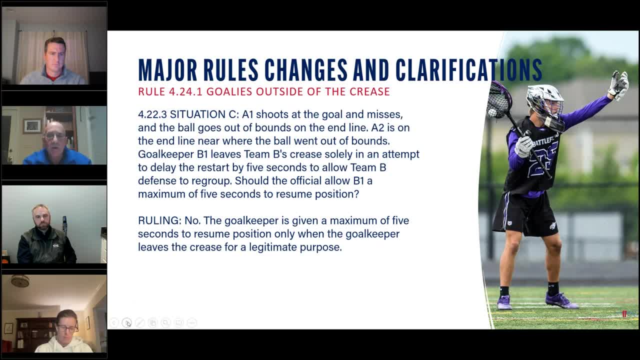 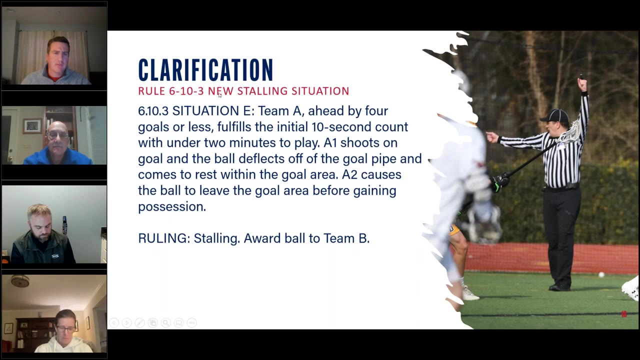 But this is what put in, Because goalies were delaying the restart to allow personnel changes. Fool me once, I'll give you a warning. Fool me twice, I'm giving you a conduct. Okay, I think this is the last one we might have. 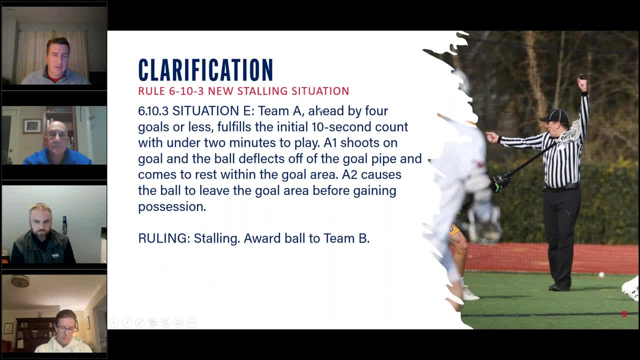 But new stalling situations? Actually, no, we have way more than that. So a team- This is when we're a point In the game two minutes or less than a team- is ahead by four goals or less, and they have. 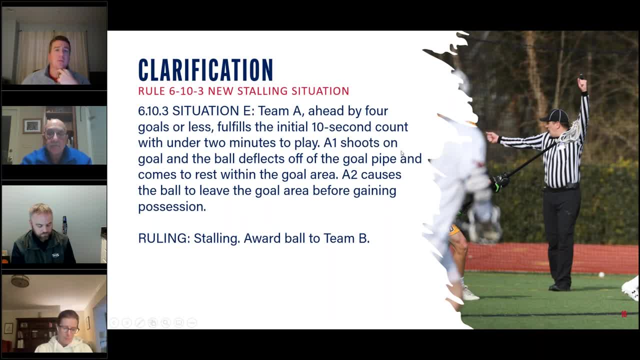 fulfilled the initial 10 second count under two minutes of play. A1 shoots the ball, The ball deflects off a goal pipe, comes to rest in the goal area and then A2 causes the ball to leave the goal area, Just ruling, stalling. 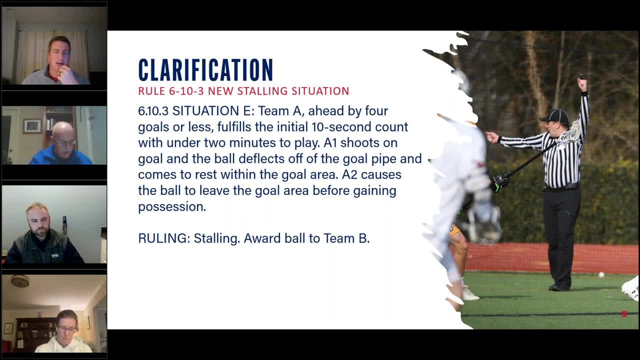 James, do you want to, or, Jim, do you want to kind of talk about the clarification that occurred? And I guess you know, maybe what was happening in the past that was causing some confusion. Yeah, Yeah, and that also, it also goes to the, to a change in a clarification from last year. 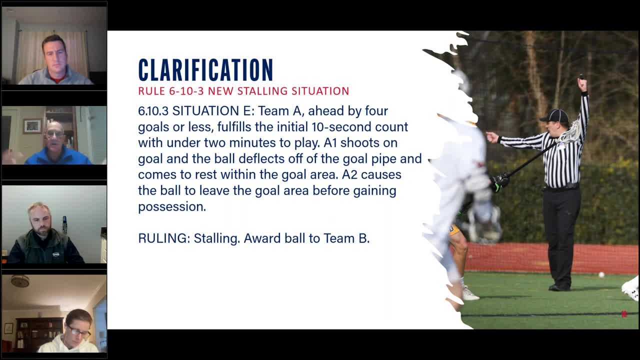 The situation we've. we've always done it. you get it in, you keep it in, But now that with the definition of a shot, a shot changes possession, a shot ends possession in a lot of situations. So now it was brought up, much like the new rule on page 77 on a 2022 rulebook, where a team 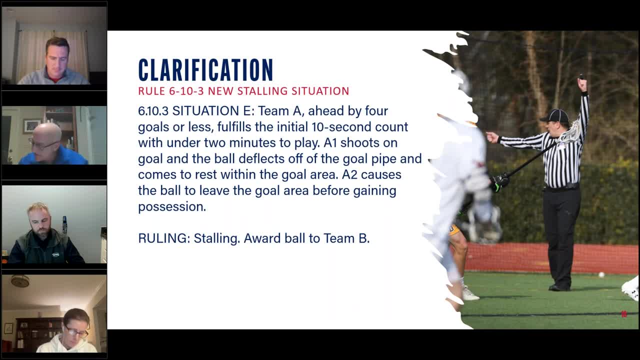 ahead by four goals. guy in the defensive end throws a Gilman, It lands in the in the box and bounces out. Is that in Uh, failure to advance or I'm not keeping it in? And for years we said, yeah, that's illegal. 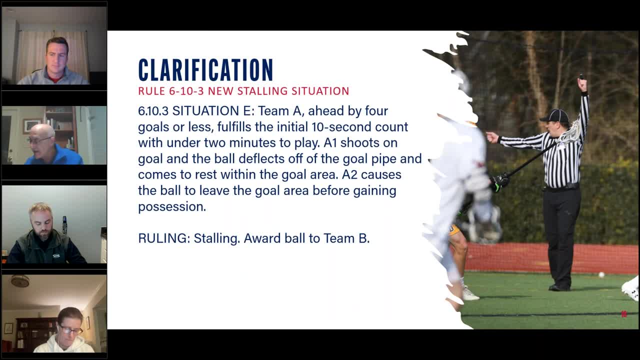 Ball goes to the other team. It was clarified last year that no, because there was no get it in. keep it in no possession in the offensive half of the field. that a Gilman pass that bounces in the box and goes out is not a loss of ball. 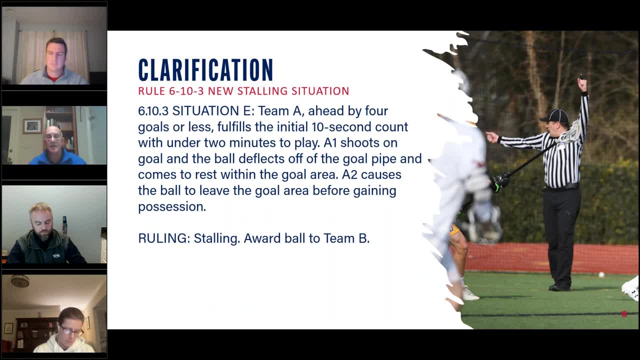 And that's what happened, And this now clarifies it, because someone said: well, wait a minute, a shot that hits the pipe possessions over. We got a new possession on it, So if I kick the ball out of out of the box, I shouldn't be penalized. 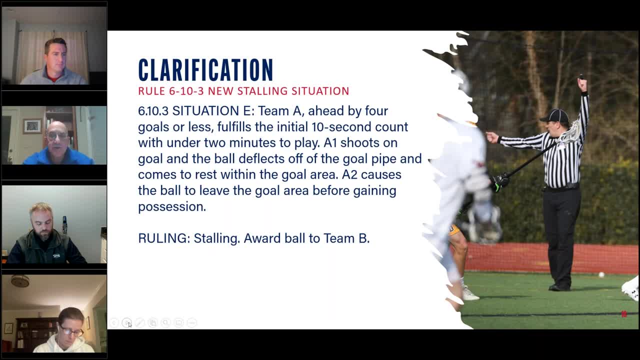 Uh, this, uh stalling situation. clarification ends that and that. if, once you've had the get it and keep it in, you've had a 10 second count uh situation and it stayed in the box, If the offensive team kicks it out of the box or causes it to leave the box, they lose the ball. 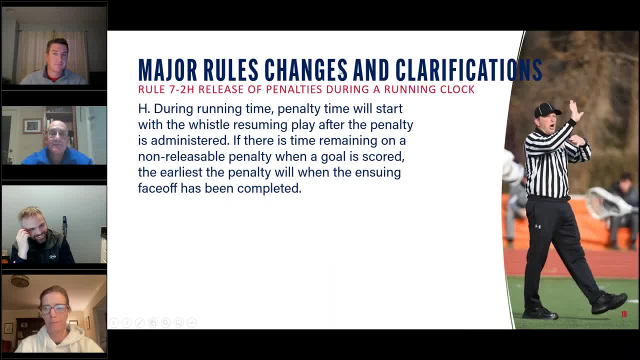 Questions, doubts, fears, Um, um, the release of uh penalties during a running clock situation. Um, Jim, do you kind of want to talk about, I guess, um, how this came up and, um, I guess, the the guidance. 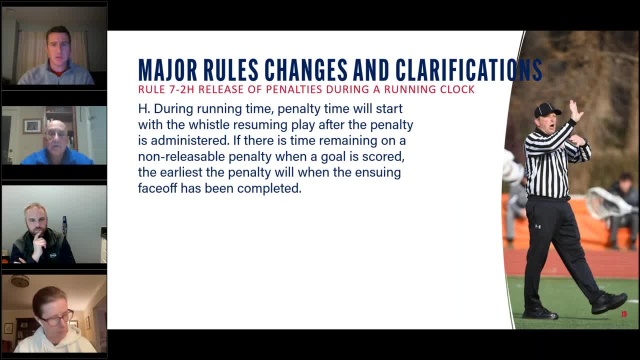 Um, again, this only has to do with running time penalties. So we're in a situation, uh, where the clock is running and it's going to be remaining running for the rest of the game. Yeah, this was something that we had in our mechanics, and and, and what we did without having a rule to back us, where you know the goal would be scored. 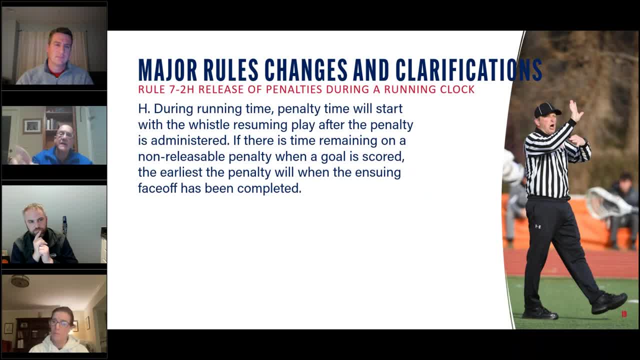 We sent it up to send the ball up the field and we tell the table and the bench penalties released on possession after the face off. but we had nothing to back that up on. And so one, Of course, you're all show me the rule. 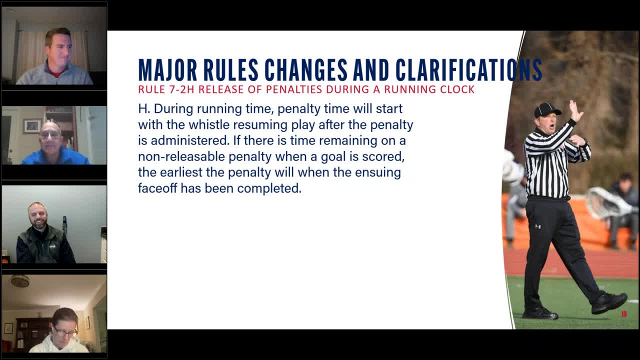 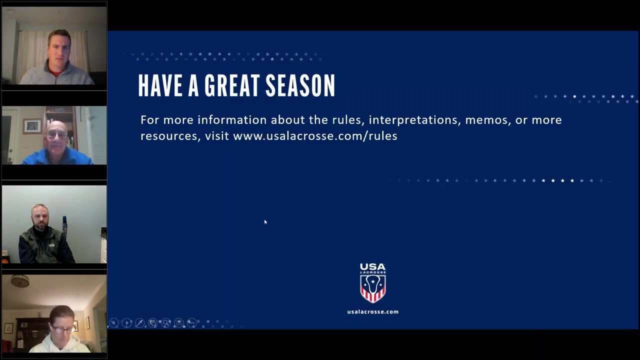 Oh, now you can, It's perfect. Great Um. any questions there? Nope, we're good. Okay, great Um. I think that that sort of does it for the presentation. I do want to take a chance to uh to to thank uh two people who um help with the U S lacrosse rules committee and the NFA. 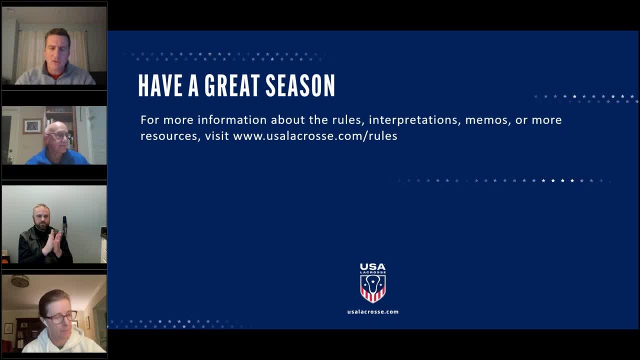 Just for A long time. Dave Simon and Walt Munzee- Um, I had the pleasure of working with both of those, uh, those gentlemen for a number of years and they did have done a lot for the lacrosse community, not just at us across in the NFA chess, but with the NCA for a long time. 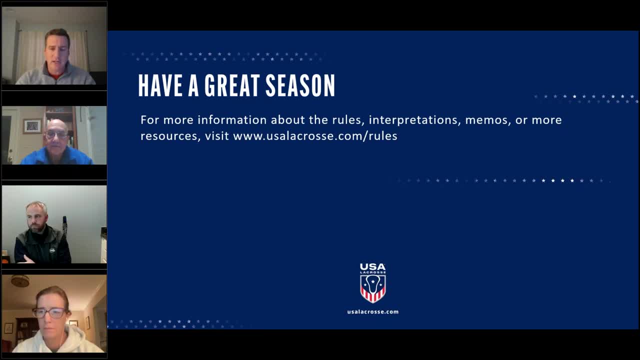 So, Dave and what, I know that you guys are out there listening and I just want you to know how much I appreciated my time with you, And I know James, um, and everyone on the call here would say the same: Absolutely. 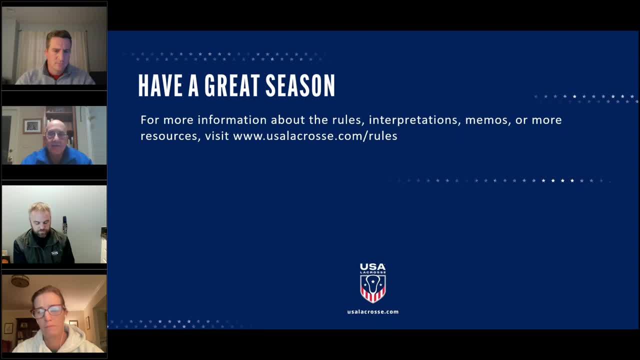 Yeah, Walt's been my mentor, guidance and days He's been my sidekick. best friends, good people, Caitlin, anything else um from the group? Nope, And we'll pull the questions that haven't been answered or haven't and we can add them into laxcon. 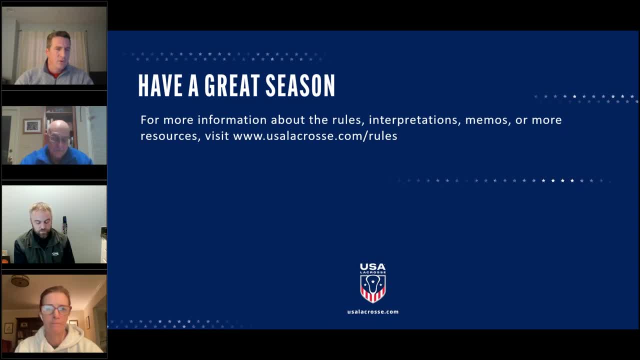 I'll send them to you all for the laxcon PowerPoint too. Okay, great, Uh. so with that, if you do have any questions, please send them in. uh to, to Caitlin, or uh, any of us that are on the the uh, the call here today. 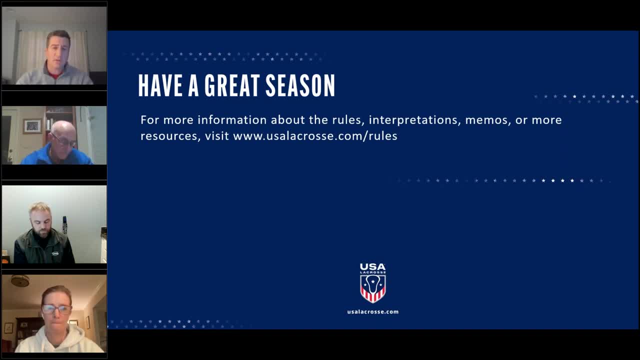 Um, Caitlin, uh, would be happy to, But we do have a couple of questions that we're going to pass them along to the committee and there's plenty of time for us to address these prior to the start of the season. 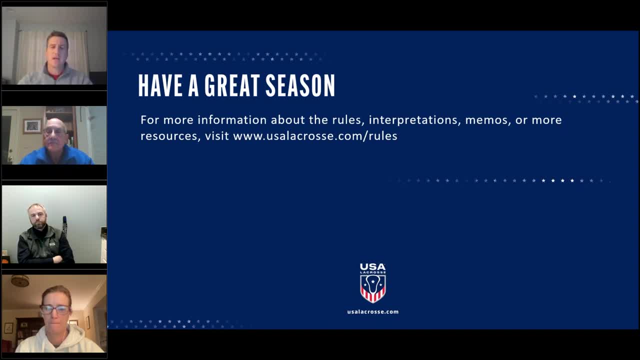 And one of the things that we want to do as well is um all the the state rules interpreters out there- James, uh, or Jim- and I want to establish contact with them And make sure that if you guys in the La Crosse community have questions, you're reaching out to your state rules interpreters. 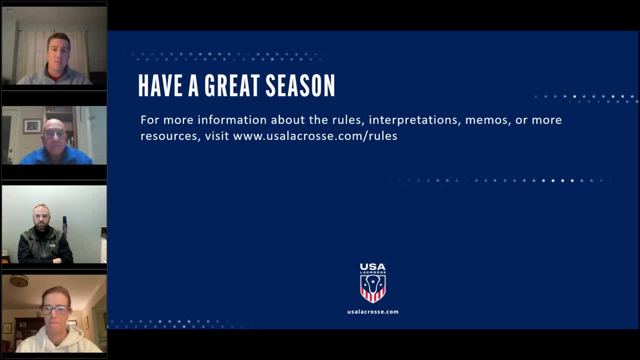 And then we want to hear from the state rules interpreters as well, so that we can find out what issues or clarifications need to be made to the rules, So we can try to bring some consistency out there. So, Uh, you'll probably be here. 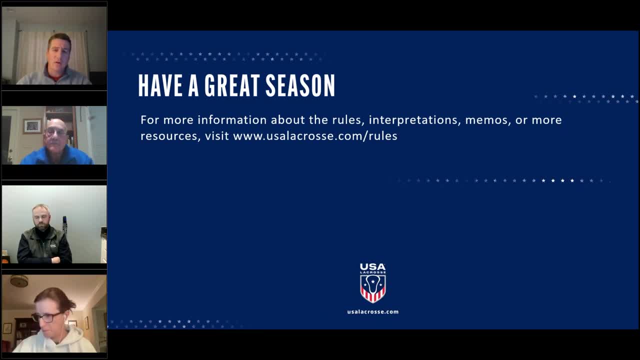 You're hearing more of that Um and and At a local level. but, uh, Jim and I are going to be looking forward to trying to reach out to the state rules interpreters to introduce ourselves. Um, I know that they probably- uh, maybe you've come across my path once or twice, um, and, and probably know who Jim is, but, um, I think it's important just to put that out there that you're reaching out, asking questions, uh, of your local association, local coaches, associations, and then reaching out to your state rules interpreters when you have questions so that we, uh, the rulemaking bodies, can get it right or know what we need to fix in the rulemaking bodies. 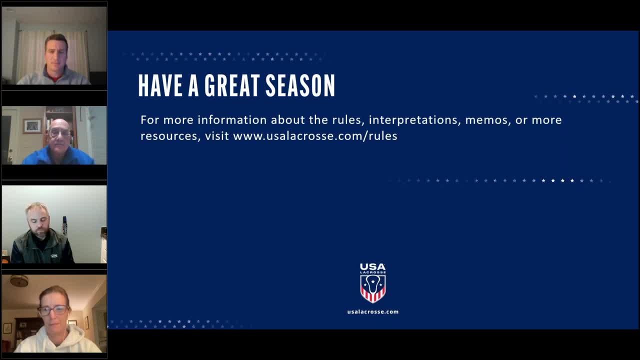 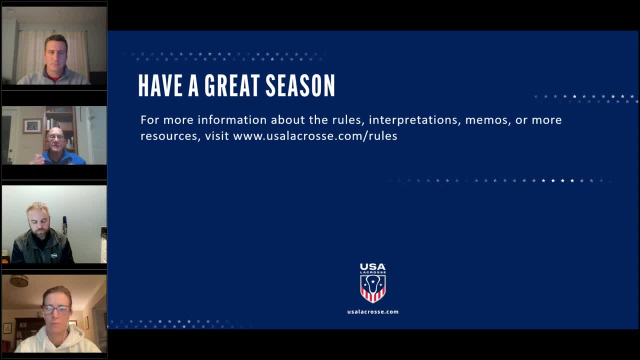 Thanks, Thanks, Right, If there's something in the rule book that you think needs to be cleaned up, fixed, get it to us. Let's start a conversation. You know, June of 2023, we're going to sit down saying how can we make this a better rule that we can officiate a better game. 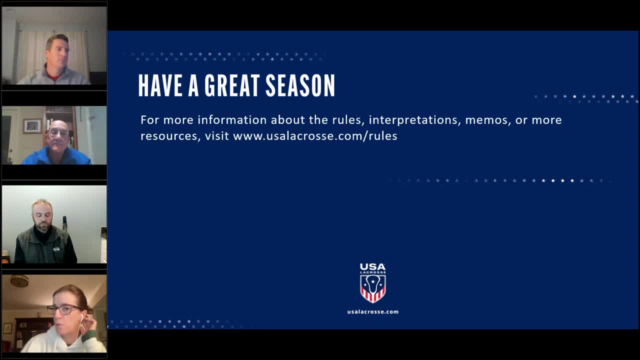 I'll just add from an administrative side One: this is recorded, So we will have this recording available. if you want to share it or reread it or go back and take notes, that will be available. And, as Rick said, if you have questions that you want us to cover at LAXCON in the larger interpretation, please reach out.